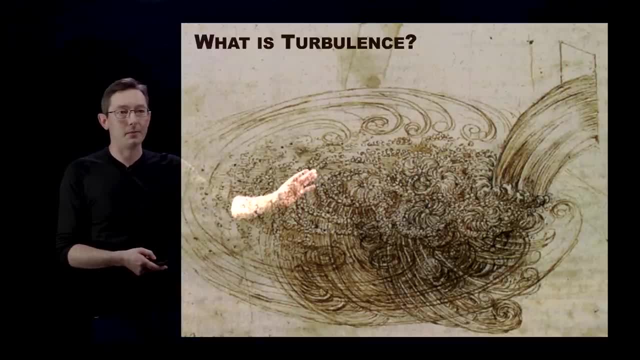 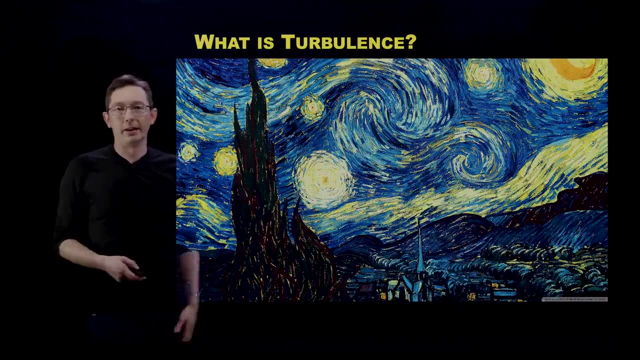 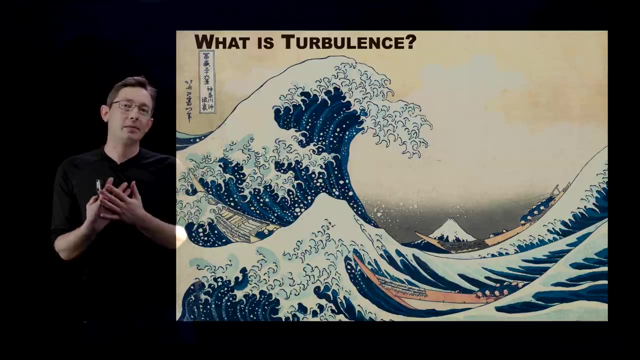 people for really for millennia. Okay, so great art has been made to try to capture the nature of turbulence. not just da Vinci. We have Van Gogh and we have the great wave. Turbulence is a part of our literature, It's a part of our very language. Some of my favorite words: roiling, churning. 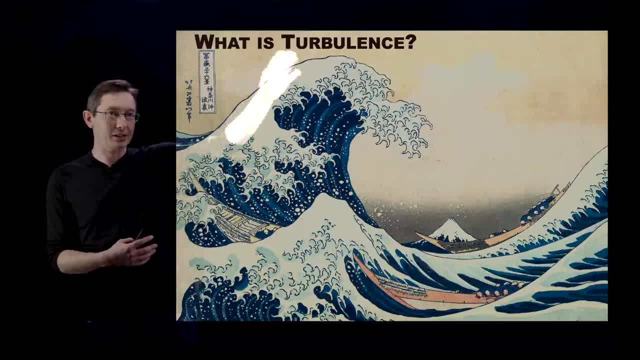 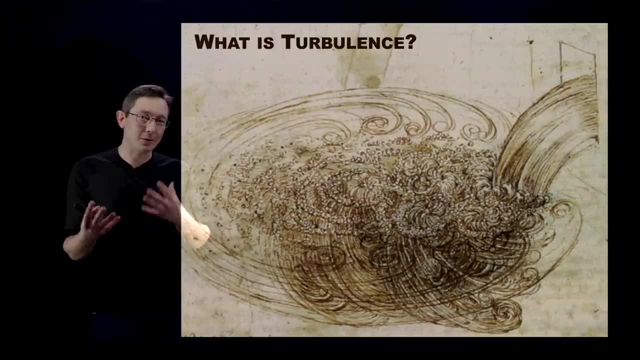 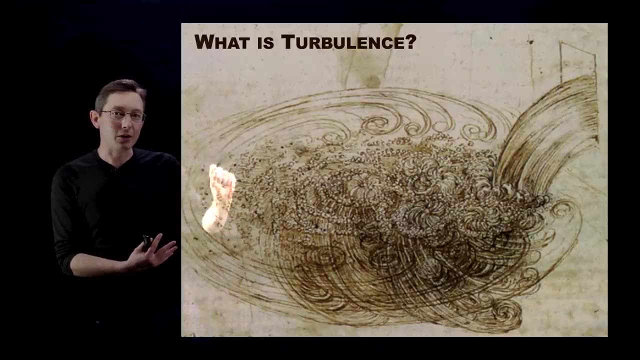 turbulent. these mean so much to us, And so today, what we're going to talk about specifically is what is turbulence? okay, And so you know, even though we have a very intuitive feeling of what a turbulent flow is and is not, it's actually very hard to pin down a single kind of unique. 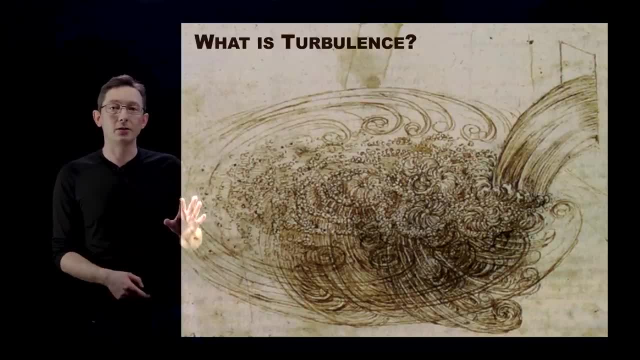 definition that we can all agree on, And so, instead of trying to do that, I'm going to bring up some kind of key features of turbulence and walk you through some examples of turbulent flows, how they're useful and how we might analyze them as engineers. 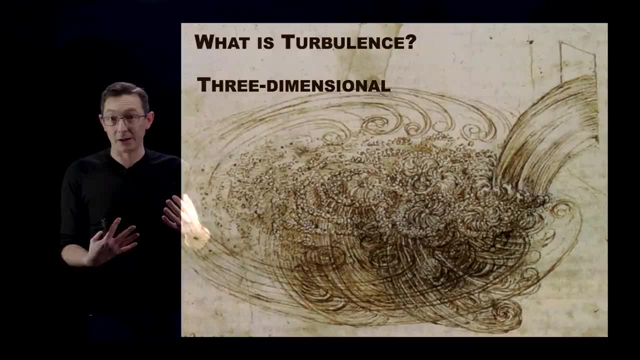 So turbulent flows generally are three-dimensional. That's one of the hallmark features of turbulence And in principle you can technically have approximately 2D flows that exhibit turbulence, but that's like a special case. So, for example, weather on the surface of Earth, we have a thin atmosphere, and so the fluid dynamics are approximately 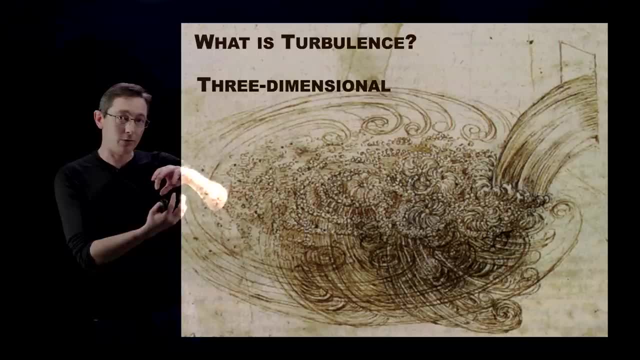 two-dimensional, But you get weird things like small vorticity adds up to make bigger and bigger vortices and form hermaphores, And so you know there's a lot of things that we can do to see what the turbulence is like, And it's also known as automobile turbulence, which is kind of 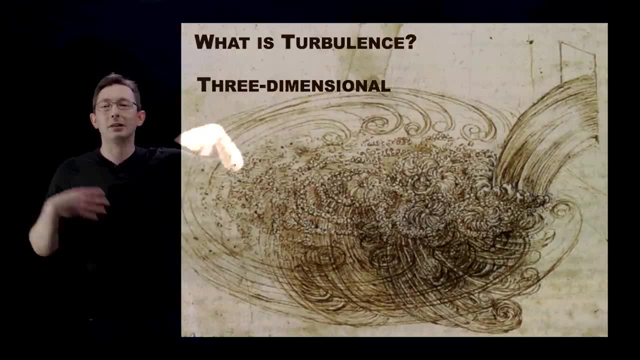 a classical three-dimensional turbulence. So when I say turbulence I really mean kind of the three-dimensional turbulence where things are spinning and roiling in three dimensions. Turbulent flows are multi-scale, okay, So they're multi-scale in space and time. 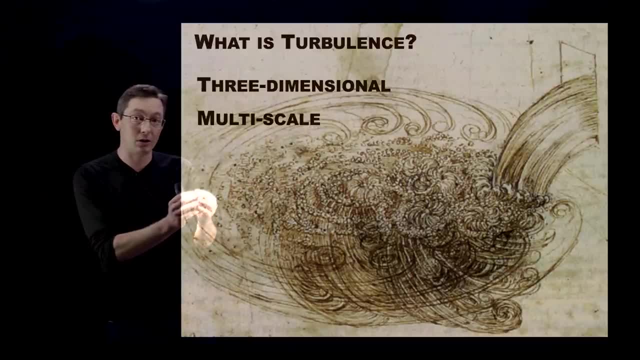 which means that there are big eddies and medium eddies and small eddies and smaller ones at infinitum. okay, And you'll notice that all of these features that I'm going to list are actually in this da Vinci painting. So you can see that all of these are actually in this da Vinci painting. 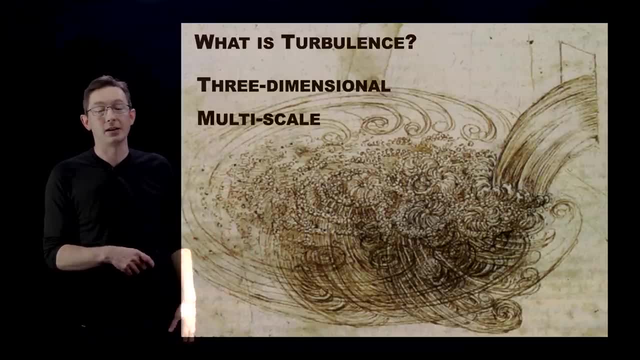 so there are many different. so let's see what we can do. to see what we can do about this, Let's see. So this is clearly kind of his attempt at three-dimensionality. It is highly multi-scale. You can see kind of self-similar patterns. 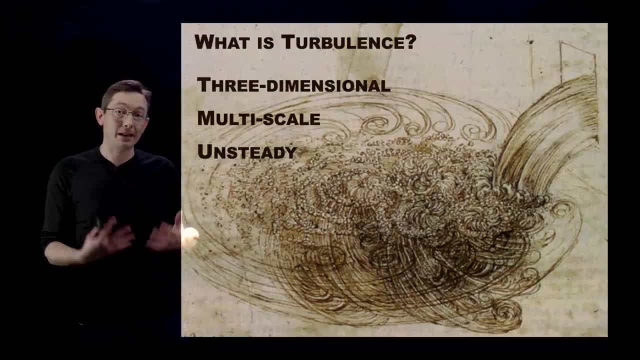 It's unsteady. Even though this is a fixed image, It clearly evokes motion. Okay, so turbulent flows are not fixed, They're not stationary, They are evolving in time, They're unsteady and They also induce mixing in the flow. So you can kind of imagine if you dropped some red food coloring into this turbulent flow. 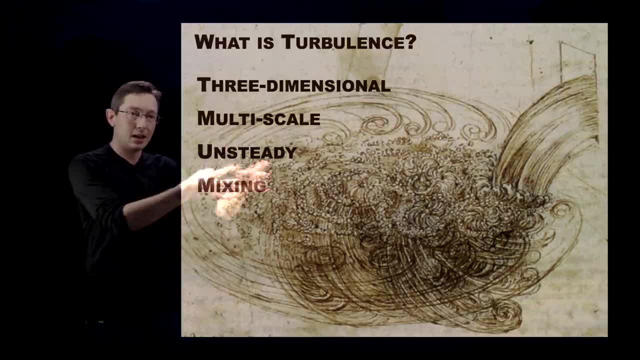 It would very, very rapidly start mixing and diffusing and kind of turn pink and then dissipate away. So these are four of the canonical features of turbulence that we're going to investigate more, And I'm gonna have a few videos in this series about what is turbulence and some examples of canonical flows, how we can analyze them. 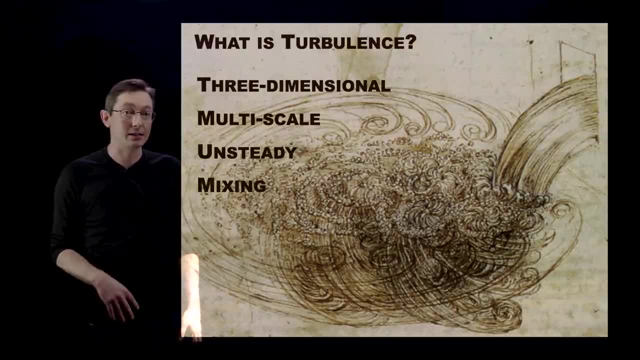 Things like that. I'll even do some kind of by hand sketches and analysis in a few of these, But this is kind of the big idea. We're going to explore turbulent fluid dynamics, which is literally all around us. Okay, and I'll point out at the outset: 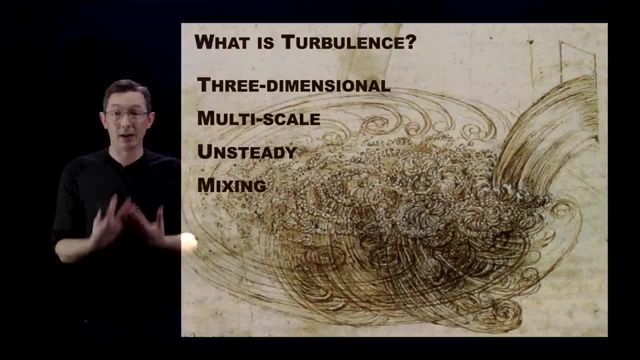 This has a tremendous amount of value for us as engineers when we design aircraft and ships and jet engines, more fuel-efficient cars and trucks and trains. Absolutely, you know tremendous applications for turbulent fluid dynamics in engineering, But I really do think that our fascination with turbulence goes. 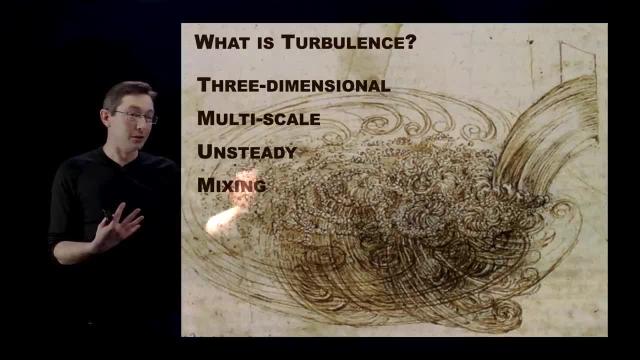 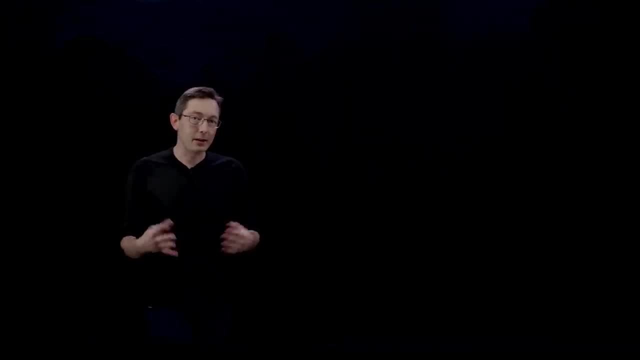 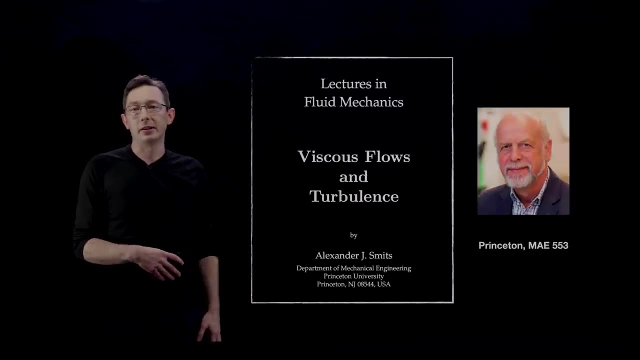 far beyond just its usefulness and, You know, is often motivated by its beauty and by the fact that it's all around us. Okay, Okay, So when I was preparing this material, I went back to a lot of the course notes where I learned turbulence, and I was fortunate to learn turbulence from Lex Smits at Princeton, and you can download these course notes for MAE. 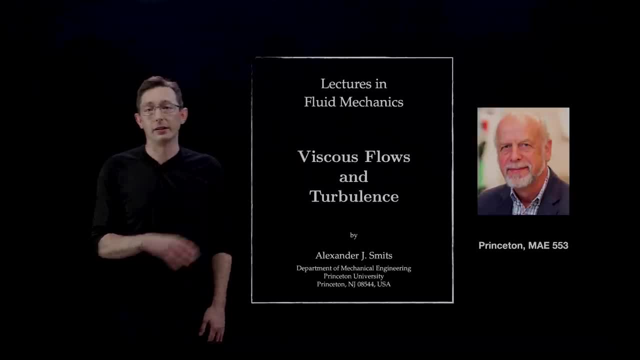 five, five, three Viscous flows and turbulence by by Lex. I highly recommend it. This is is absolute gold and a lot of what i'm going to pull from in these videos was, you know, out of this, this book. so i highly encourage you to check this out, because this really is a unique perspective. 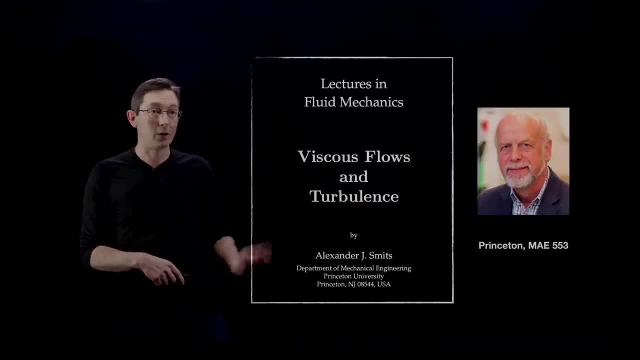 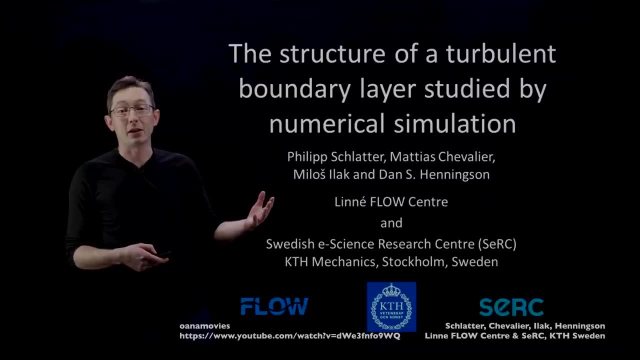 from one of the absolute foremost leaders in the field. okay, good, so we're going to start talking about about turbulence, and i want to just start off with some, some videos and some pictures just to kind of, you know, get you thinking about what we're. what we're talking about. this is one of my 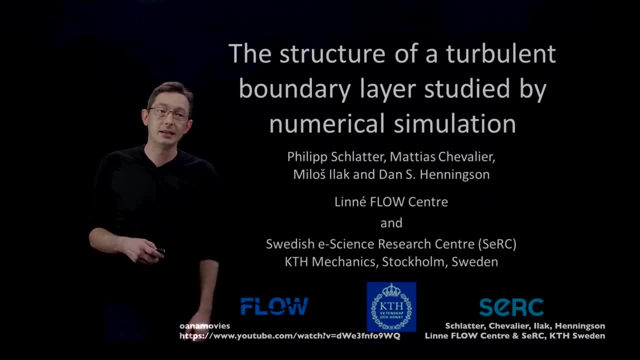 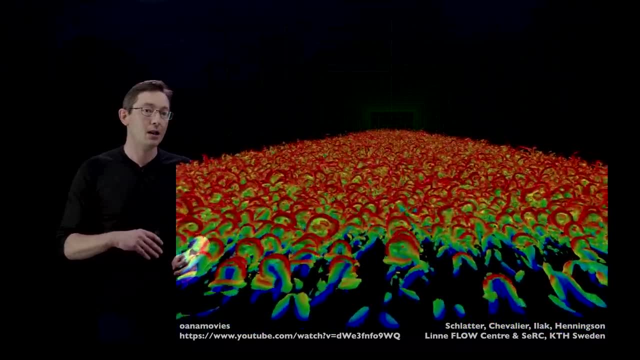 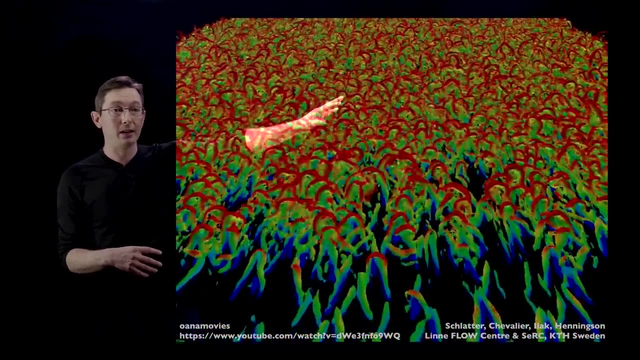 favorite videos by colleagues at kth in sweden, and so this is going to be a simulation of a boundary layer and you know, some of you have seen this in my videos before, but this is a a very, very high fidelity numerical simulation of a developing a boundary layer flow. so basically, think of the 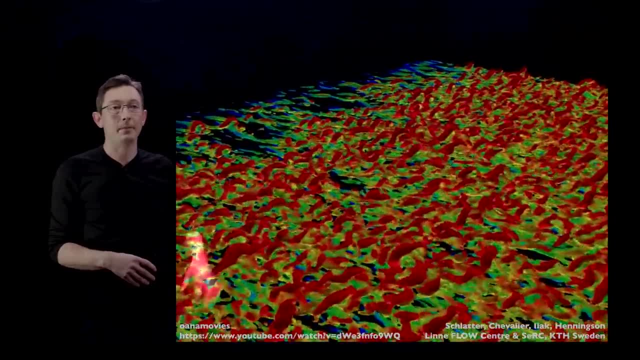 flow over a wing, as that wing is going through the air. that's what this is trying to simulate, or maybe the flow over the top of your car or train, and what you're going to want to do is you're going to want to think about what you're going to. 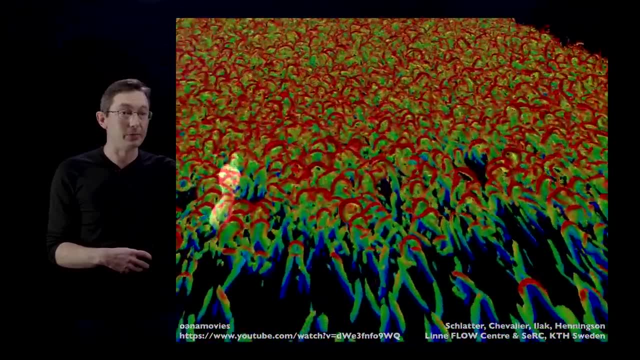 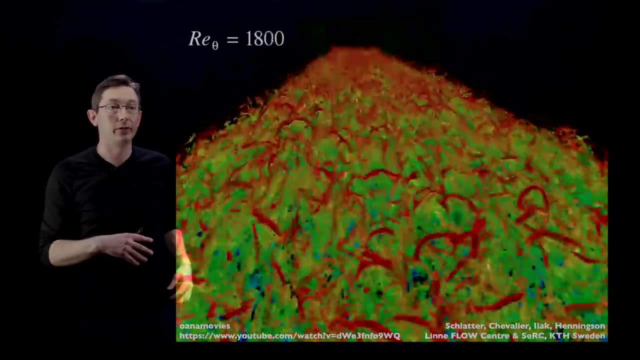 see here this has all of the features right. it's three-dimensional, it's unsteady, it's evolving in time, highly multi-scale. look at the vast, vast range of scales that are captured by this turbulent flow and clearly it's mixing, if you started out as a little upstream particle. 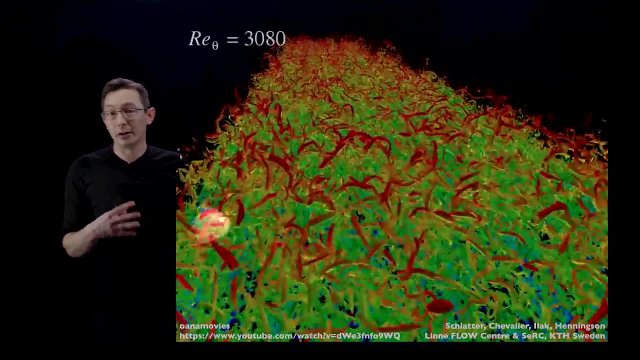 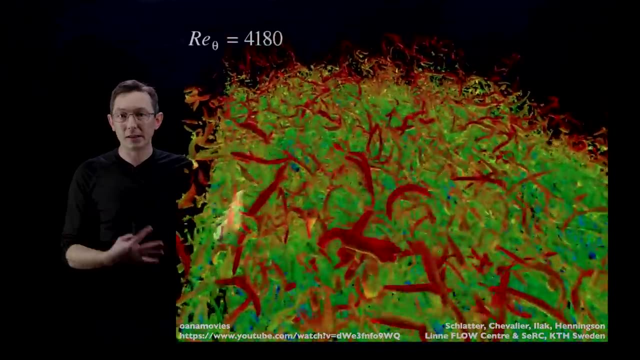 you'd be bouncing around between these eddies and after you know long enough, you wouldn't know which way you end up. okay, so this is a great kind of visualization of a turbulent flow that we can have in our mind for the kinds of things we might care about. 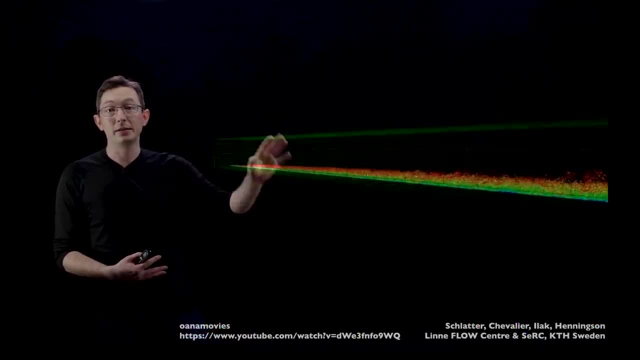 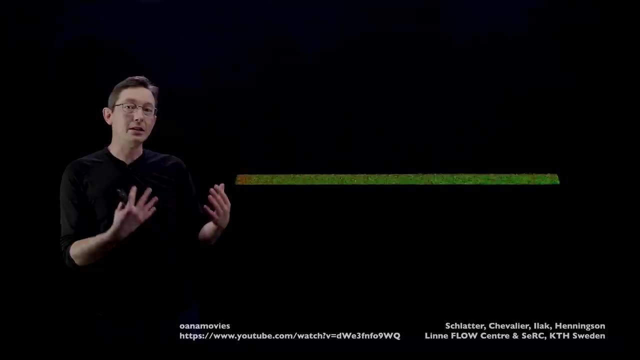 and simulating and understanding and modeling these flows is very important. again, if i'm designing an aircraft or i'm designing a wing for an aircraft, i need to know what the drag coefficient is going to be for that wing. i need to know what the skin friction as i go through. 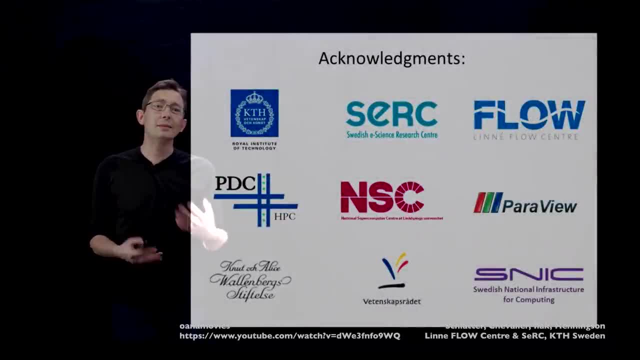 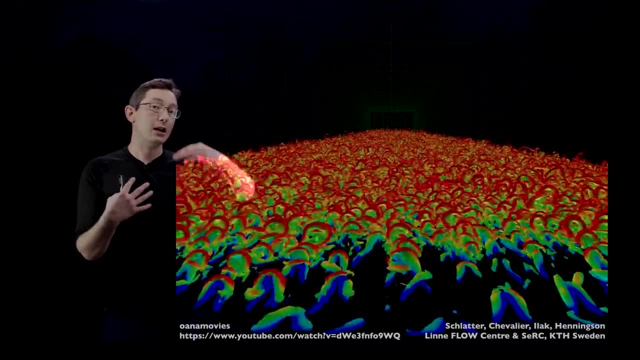 the air or through the water is going to be and i need to be able to know how that changes as i increase the speed of the flow, decrease the speed of the flow if i change the curvature of the flow by the 67- deflection of the ultrasonic, the transfer of the air softener, the curvature of the 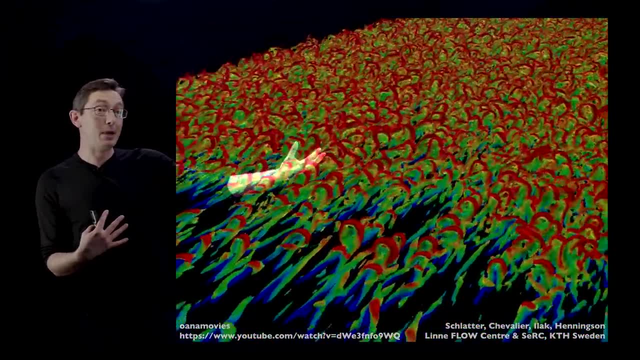 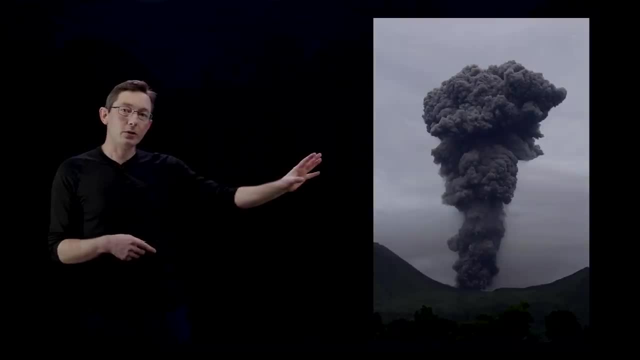 air foil, things like that, and so it's very, very hard to model these things, and this is currently an open challenge in engineering is finding better ways of modeling and optimizing and controlling these, these turbulent flows. so another cool example- and again i i kind of got this uh. 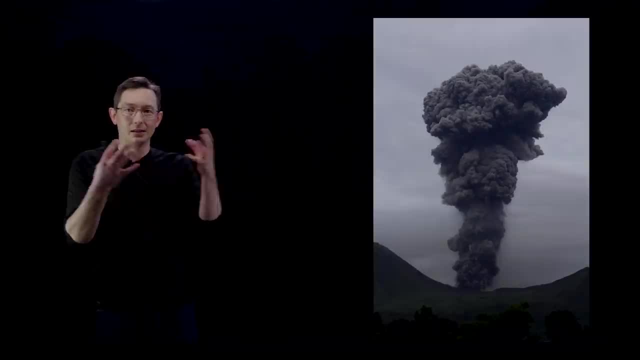 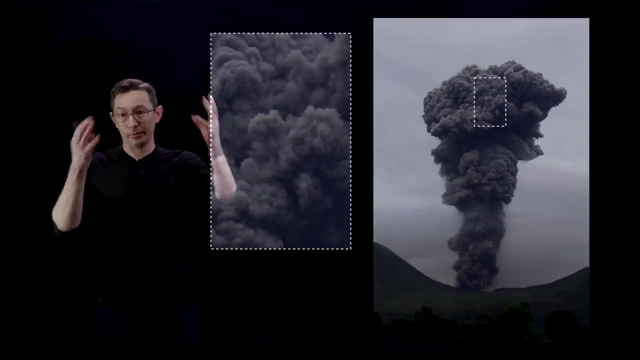 this idea from from lex smith's. you know, when you see a turbulent flow, you'll know it because it's going to have this multi-scale structure that the more you zoom in, zoom into, you're going to see more turbulent structure and more kind of fine details and 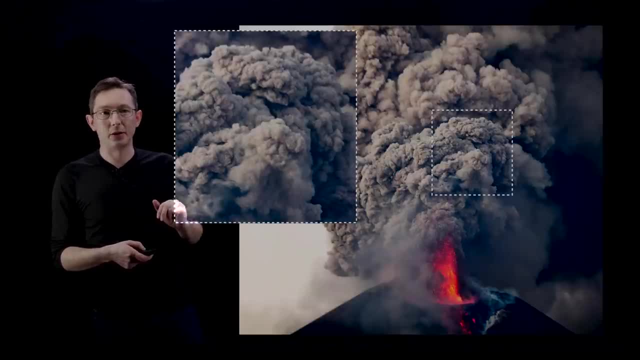 resolution. another cool example is this: this volcano erupting. you pick any spot and you zoom in and you're going to see more roiling and churning and turbulence. and actually one of the things i remember uh lex saying was: you can kind of tell how high budget a hollywood movie is. 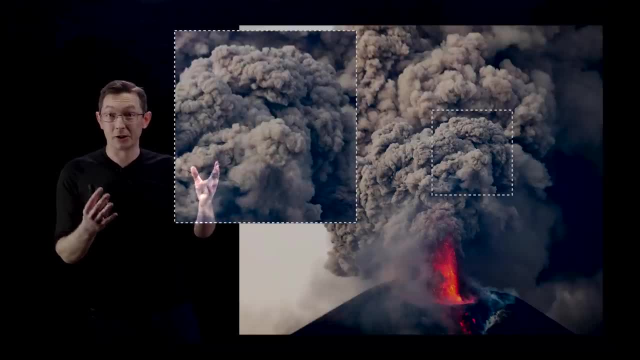 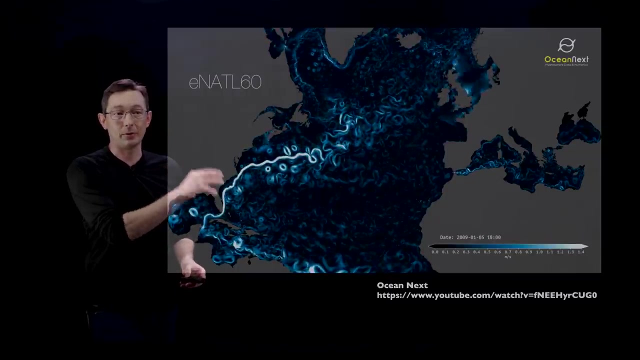 based on how many scales are in their turbulent explosions. okay so, and you know now, i can't watch any action movie without looking for that multi-scale structure, and i bet you're not going to be able to either. okay, another example. i really like this ocean. next project you can google. 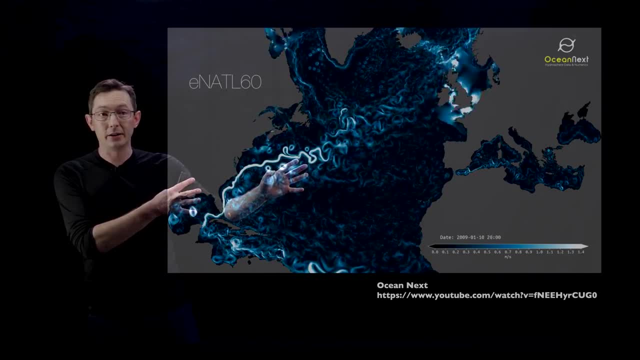 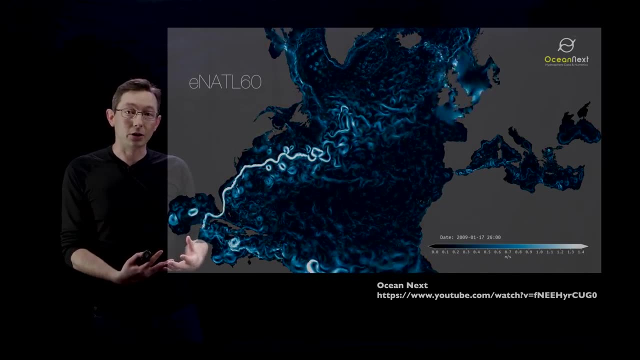 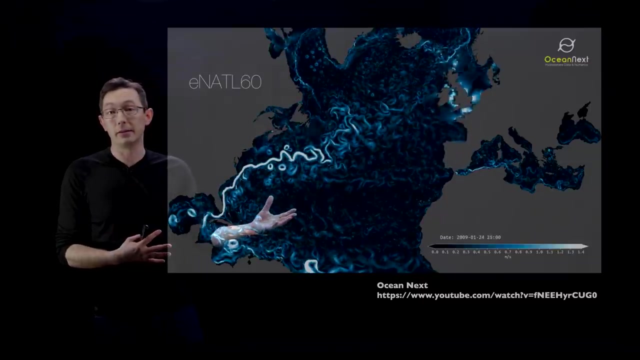 and download data and kind of follow what they're doing. but you know climate, the earth's climate, the ocean currents and the atmospheric patterns are highly turbulent. they mix and kind of transport and they're very, very important for us to better understand mixing and transport and dynamics in. 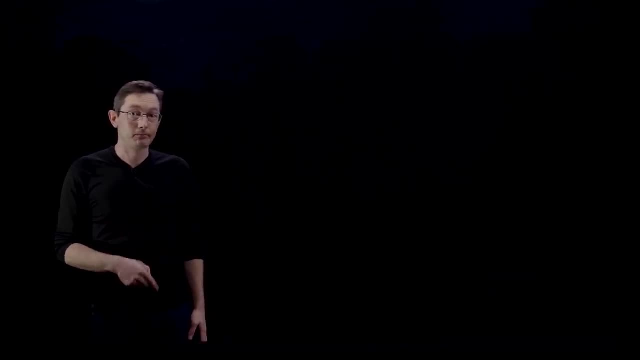 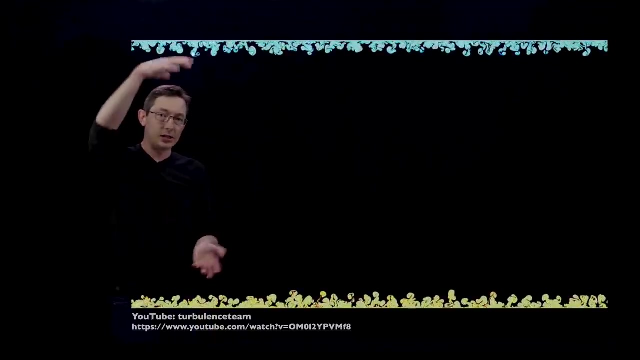 those turbulent systems as well. good, now i also want to give an example. one of my favorite examples is this rayleigh bernard convection flow, where you have a hot plate on the bottom and a cold plate on the top and you can see that just from this thermal instability you get this kind of rising of the warm. 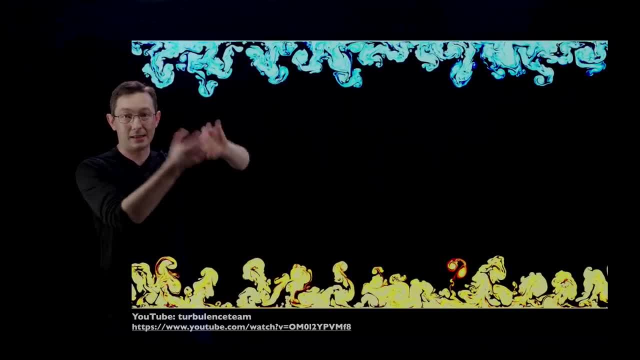 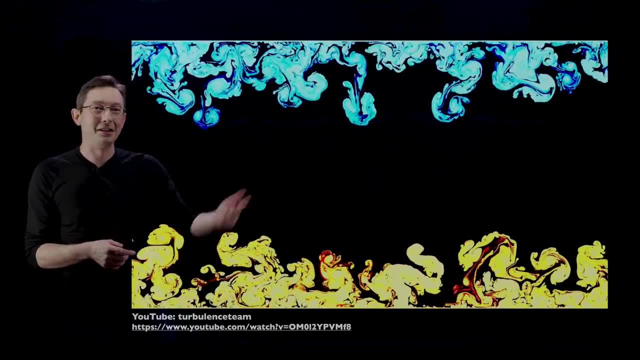 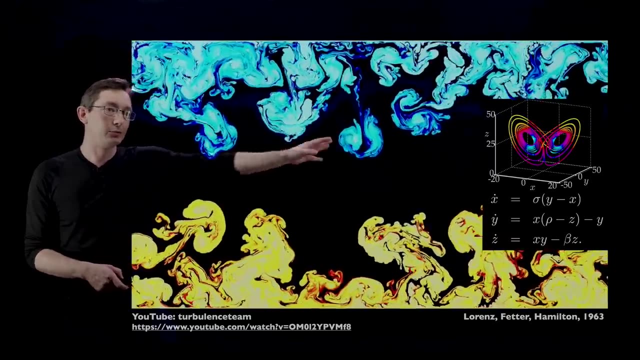 air and eventually you're going to see this start to mix in a pretty chaotic fashion. now, this is not three-dimensional, so, but it is unstudied, multi-scale, and and mixing, and this is one of the original problems that motivated chaos theory. so uh, lorenz in 1963 was studying this kind of rayleigh. 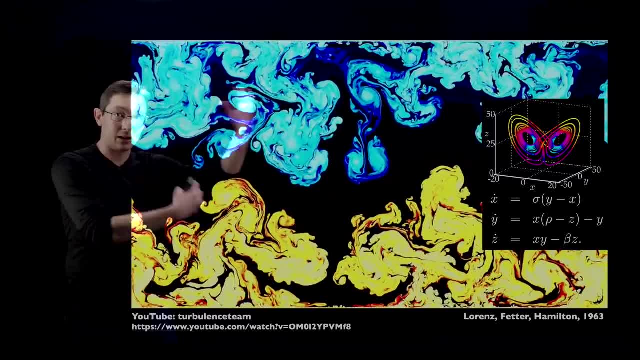 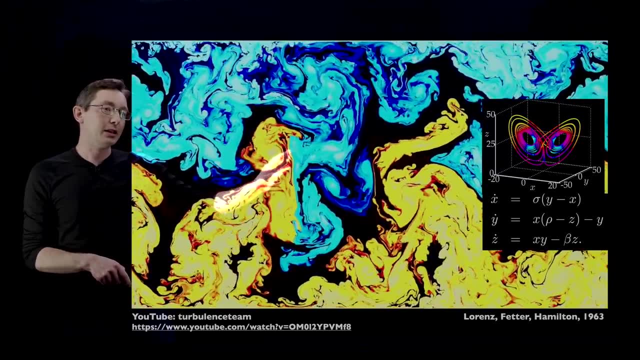 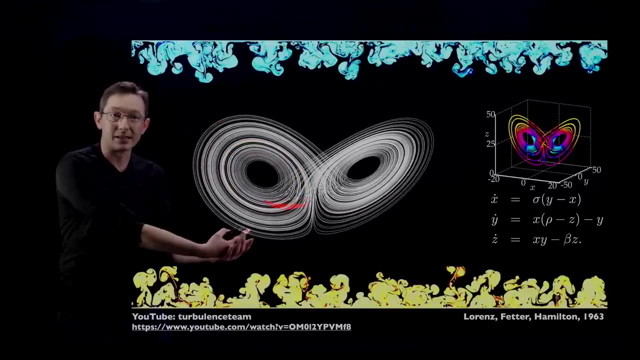 bernard convection flow, trying to model the chaotic, uh churning and overturning of these large, large eddies in this domain, and so i think there's always a very deep connection between turbulent fluids and chaotic dynamical systems, and that's kind of where this mixing idea comes from. i started with this red. 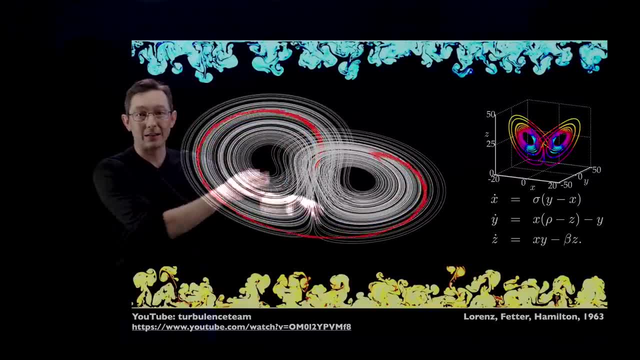 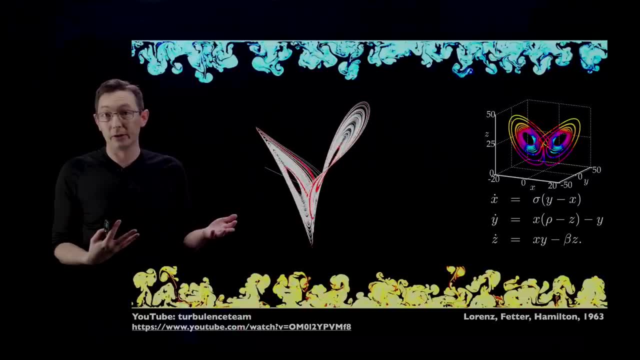 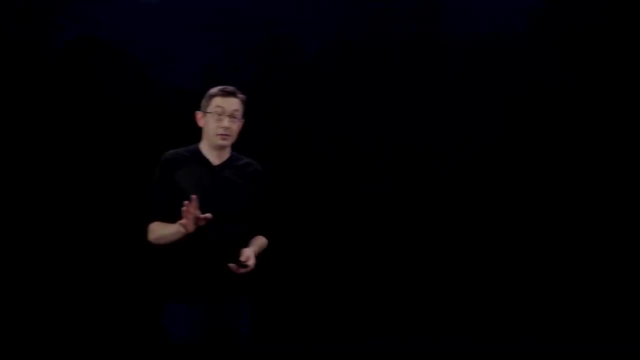 blob that was coherent after a very short amount of time. in this chaotic system, it's going to mix and spread around, and that's what happens to particles in turbulent fluids as well. okay, and i'll talk a lot more about chaos, uh, in future, in future videos. 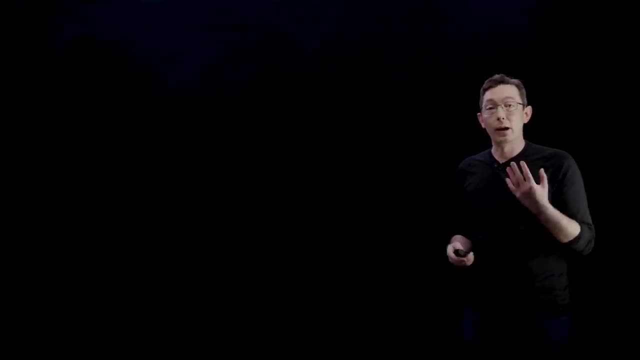 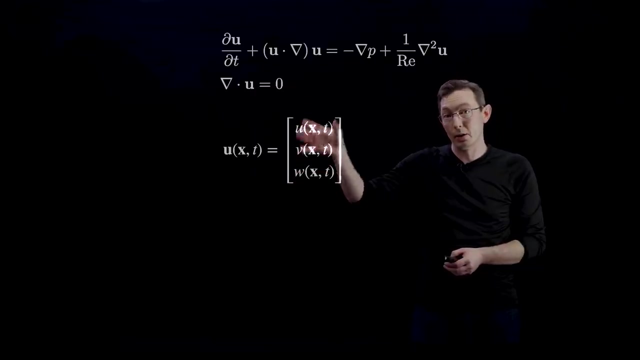 so now i want to get a little bit more into the mathematics of kind of where this comes from and how do we analyze these flows. and so we're going to start with the incompressible navier stokes equations, and i'll point out that this bold u that i'm dealing with here is really a three component. 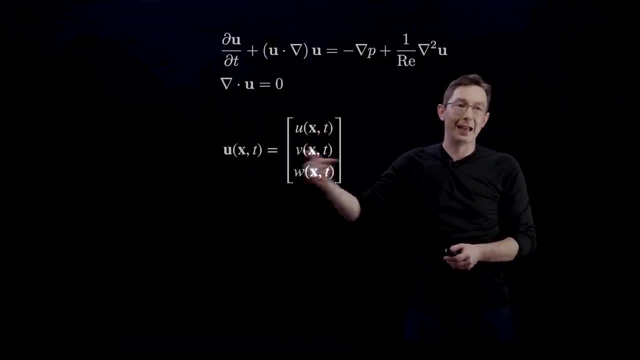 velocity field. so u, v and w are the x, the y and the z or z component of the velocity field, and that's defined everywhere in space and in time. okay, so u is, a is a vector field and these are the governing navier-stokes equations. 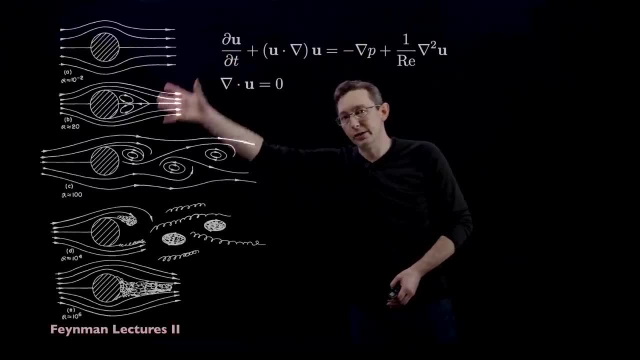 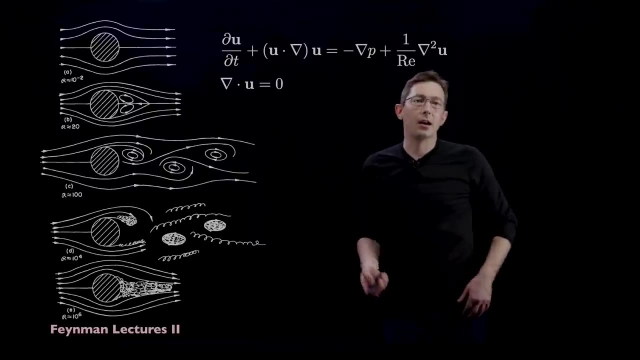 now, from these equations you get a whole range of interesting flow phenomena just by speeding up or slowing down the flow. so we have slow flows up here and fast flows down here, and you get this rich range of dynamics as you increase the flow velocity. i took this from the, the feinman lectures, and it turns out that this, uh, this range of complexity is 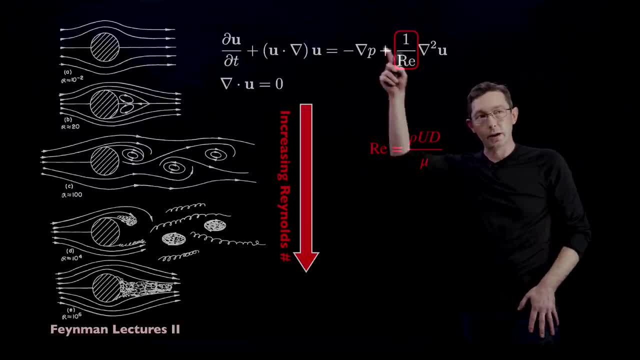 controlled by this number, here called the reynolds number, so one over the reynolds number. and the reynolds number is essentially a product of the fluid density, the velocity of the flow, the diameter of the of the sphere, in this case, or the cylinder divided by this dynamic viscosity. 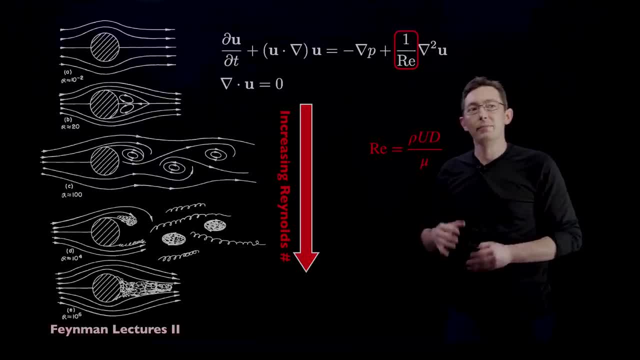 quantity. and so you, you multiply and divide all of this up and this one number tells you if you're going to have a simple flow or a very, very complex flow. okay, so increasing either the diameter d or the flow velocity will make the flow more turbulent. okay, and decreasing those makes it more laminar or less turbulent. 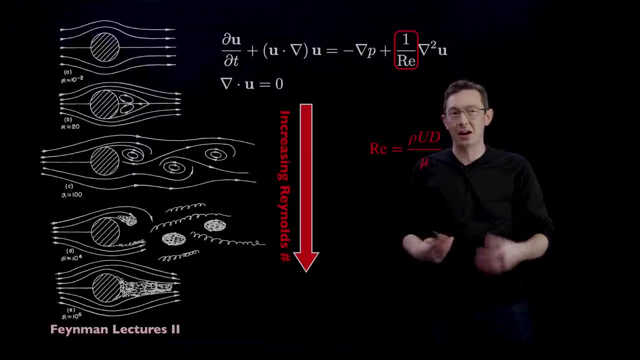 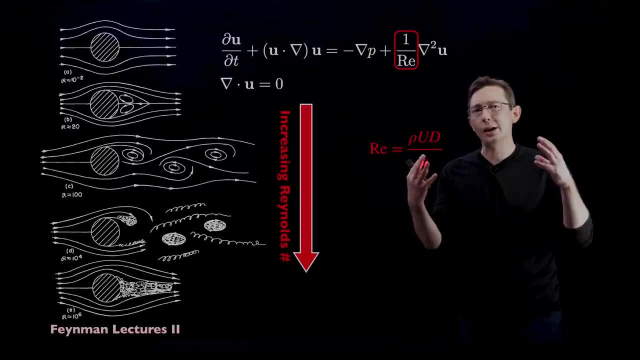 and this turns out to be an extremely useful concept- that increasing the reynolds number generally corresponds to an increase in complexity and turbulence and multi-scale ness of the flow. and in fact the reynolds number can somehow be thought of as the ratio between the largest scales in the flow to the teeny tiniest scales in the flow. so if i have a 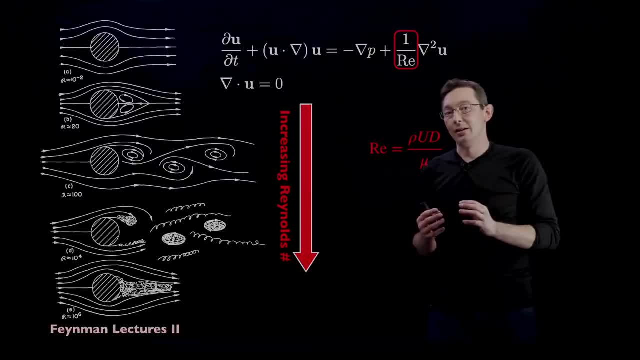 reynolds number of a million, i'm going to expect eddies- uh, you know that are a million times bigger than the teeny tiniest eddies, or or swirls or vortices in the flow. okay, that's just a kind of. 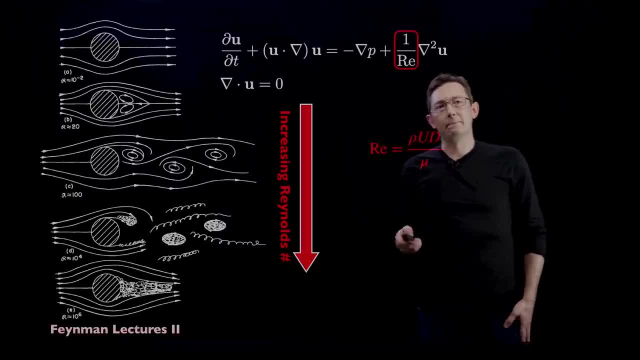 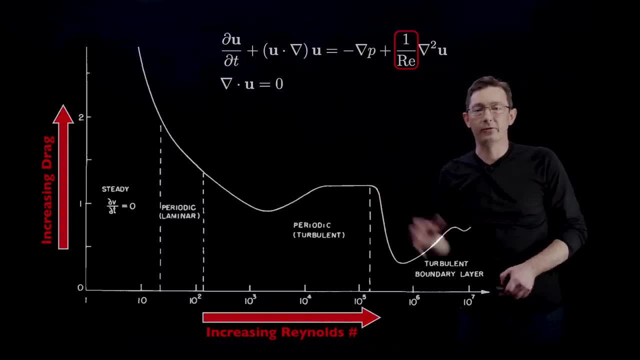 a rule of thumb, but a very, very useful one. okay, good, um, you can also plot the drag coefficient versus this increasing reynolds number. so this is a curve- uh, i believe it's called the reynolds number, i believe from nasa- and you can see that as the flow field changes as you get this kind of. 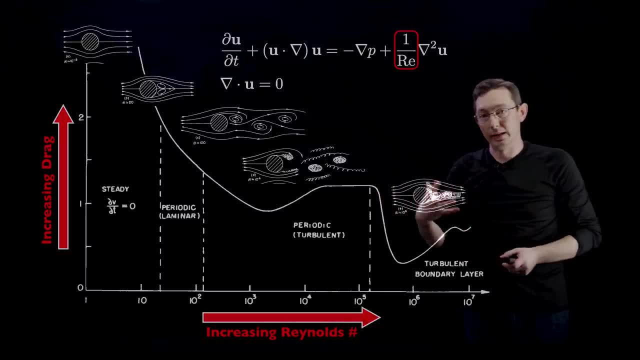 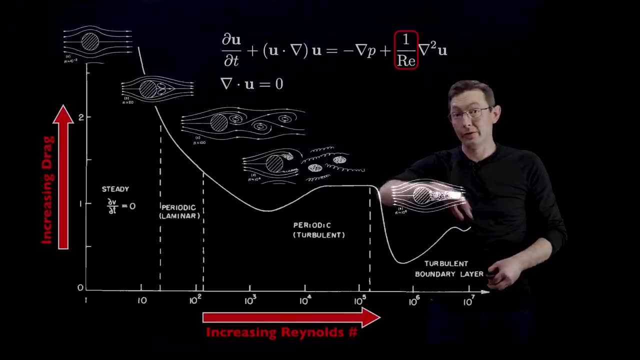 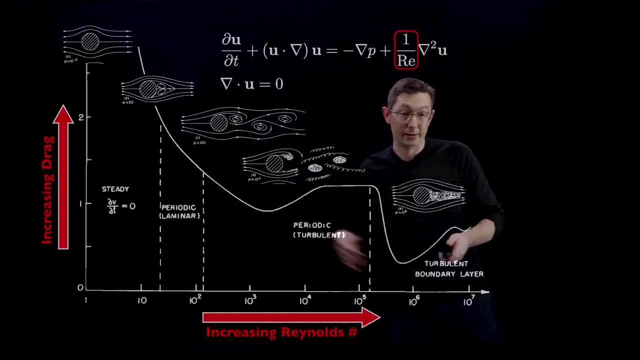 increased complexity from the turbulence in this flow field. as you increase the reynolds number or the flow velocity, you can see that you get a wide, wide range of drag forces on that cylinder. so you get, you know, huge range of drag forces just by changing the flow velocity. 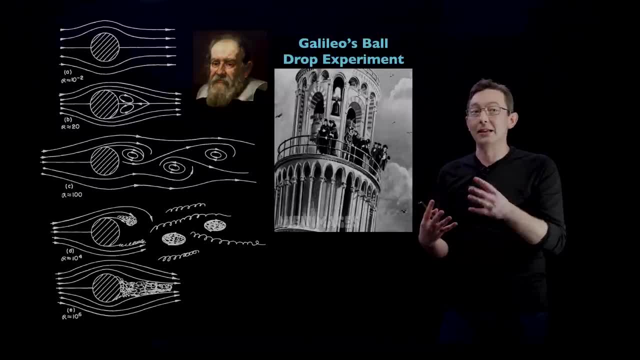 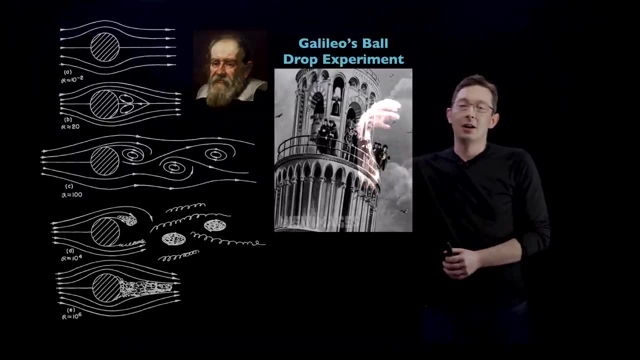 now i can't, uh, help myself. i have to relate this back to the galileos uh, famous ball drop experiment from the leaning tower of pisa. you can now picture dropping this ball from this tower as it accelerates from gravity and speeds up. it's going to transition. 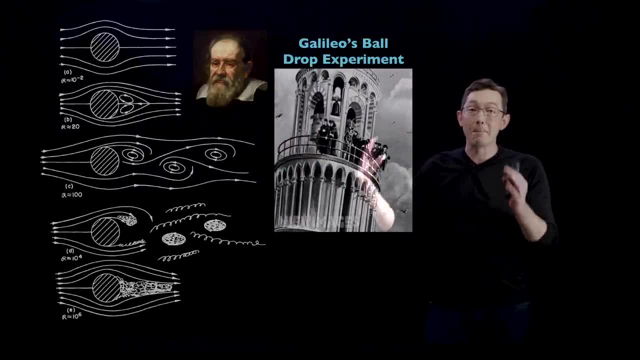 through all of these different flow regimes and experience massively different drag forces at every stage of its fall, and so, technically, its acceleration is not going to be, you know exactly, a constant due to gravity, because it's going to have this very unsteady drag force due to these turbulent forces, and it turns out, you know, this is actually. 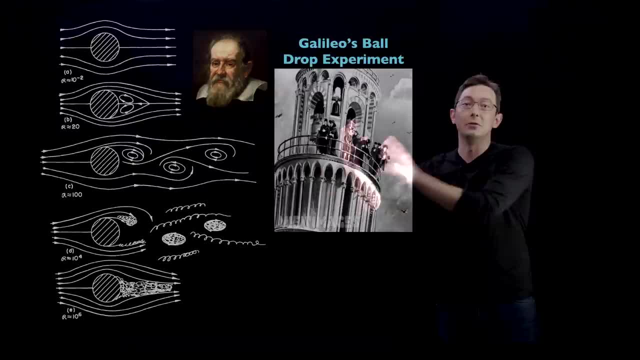 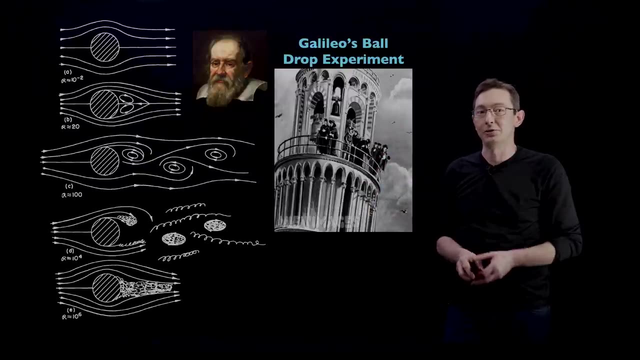 pretty consistent with the older aristotelian view of. you know, a ball's trajectory is going to depend on its mass or its density or its ability to resist these unsteady turbulent forces. so just kind of an interesting connection. if you think about that ball drop experiment, it's actually not so obvious that gravity would be a constant if you did it. you. 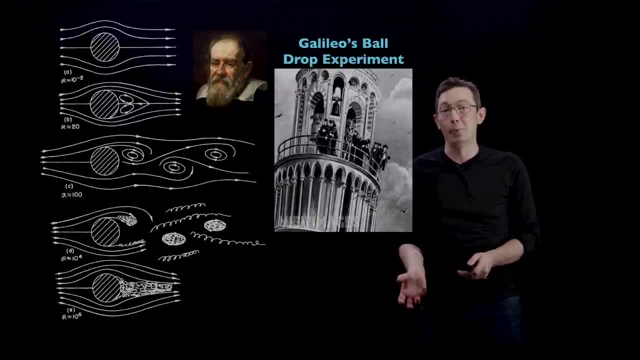 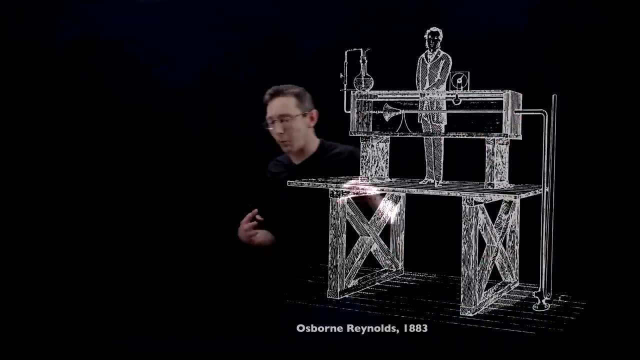 know naively now, if you drop a heavy enough ball like a bowling ball, maybe these are kind of negligible forces. okay, good, so i want to go back. why do we call this the reynolds number? so that that number, that reynolds number that controlled the turbulence from laminar or smooth? 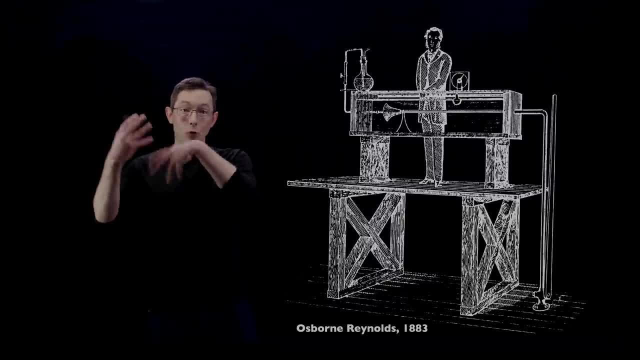 solutions. laminar kind of means layered, and so that means not roiling, not unsteady or or turbulent. and it turns out that reynolds- osborne- reynolds- in 1983- was doing experiments in a pipe. so pipe flow is one of the most important and oldest engineering. 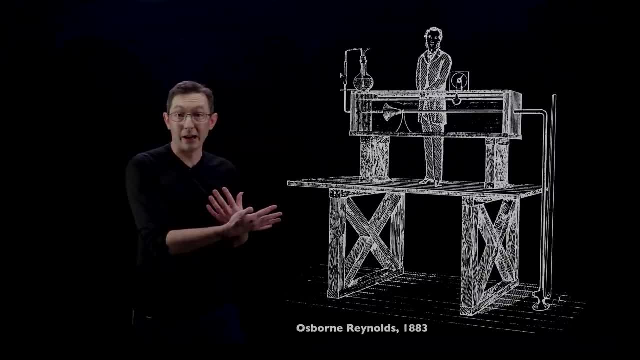 applications of fluids is literally just pumping water through pipes makes sense. you, you know how big of a motor do i need to pump all of that water through all of my city streets, okay, and to pump all of the sewage out, and so pumping water through pipes has always been important and osborne. 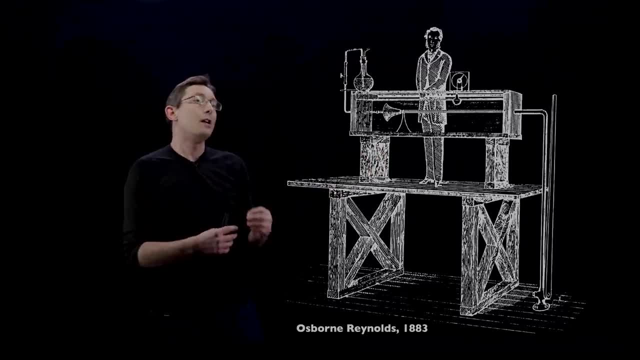 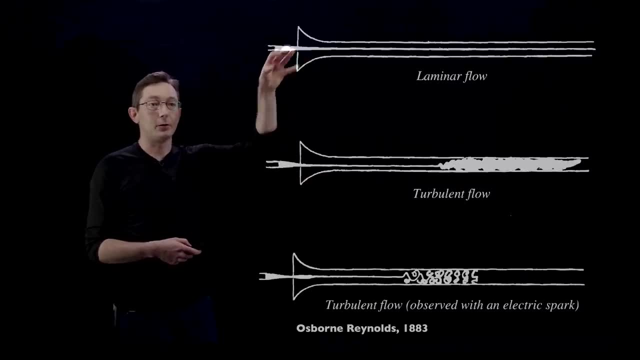 reynolds was studying, you know, the flow through these pipes and made a very interesting observation that as he increased the flow velocity he had these very different regions or characteristics of flow, from laminar flow, again layered, or very kind of steady flow, all the way down to these. 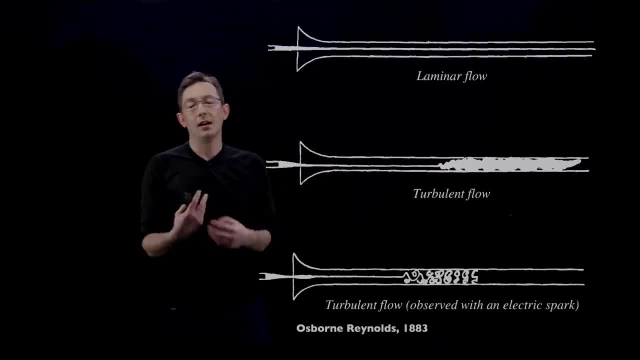 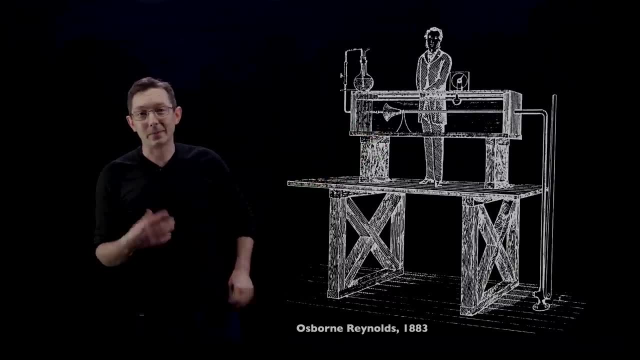 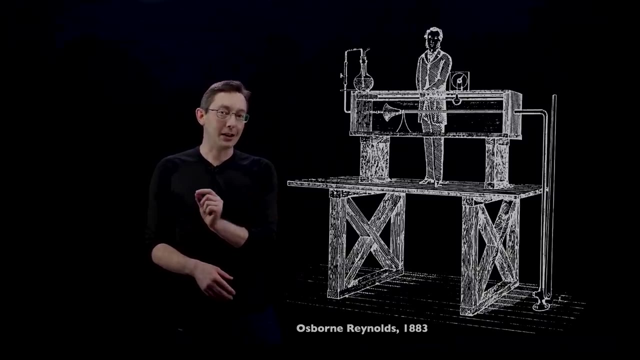 turbulent flow scenarios where the flow was kind of roiling. you know what you picture as turbulence. now i don't think this picture does. does this experiment justice? because in this picture he looks very calm and composed. but you can imagine if you were trying to do an experiment of pipe flow and you were trying to get a smooth. 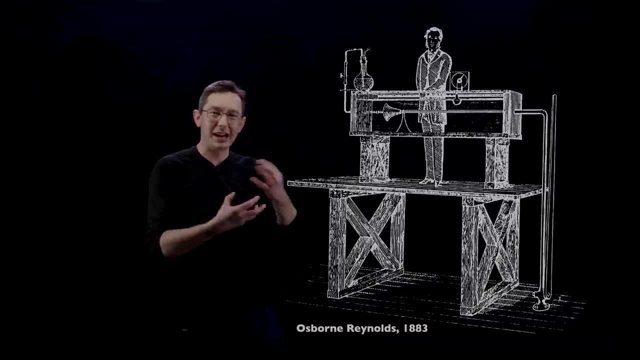 solution to collect whatever numbers you cared about and it was getting turbulent and roiling, you might have thought that something was wrong with the experiment, that you weren't doing it carefully enough or that maybe your flow wasn't well conditioned going in. so i think in this picture he really should have been biting his nails and pulling his hair out. but 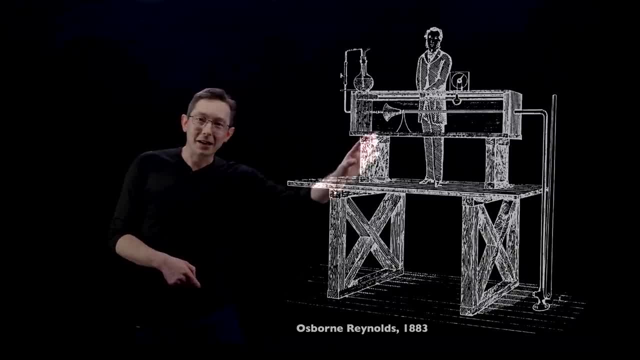 you know, this is a little bit more composed and actually, uh, you can go and see this uh original apparatus at the university of manchester. so it's still there and it's still kind of on display, which i think is kind of cool. but so a long time ago we've known that there were these transitions as you increase the flow. 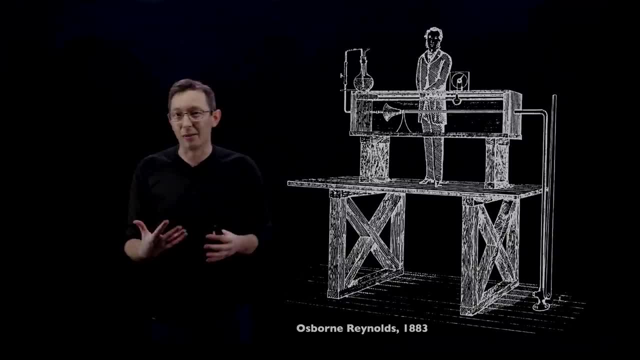 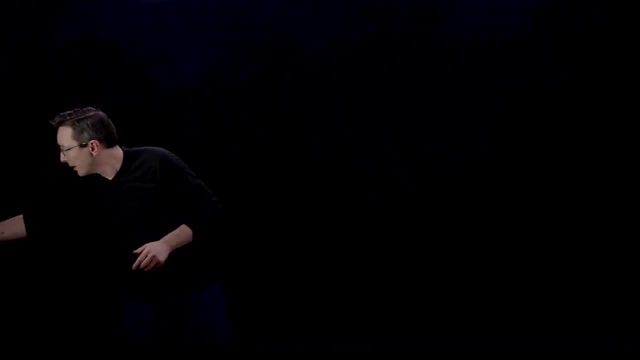 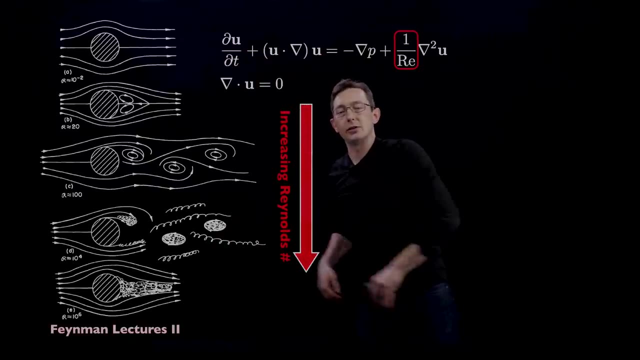 velocity, you can trip the flow into these very complex, disordered turbulent solutions, okay, good so. So let's go back to kind of this picture here. So as we increase the Reynolds number, we get more and more complex turbulent flows. But what I want to point out here is that this flow here in the middle, this kind of 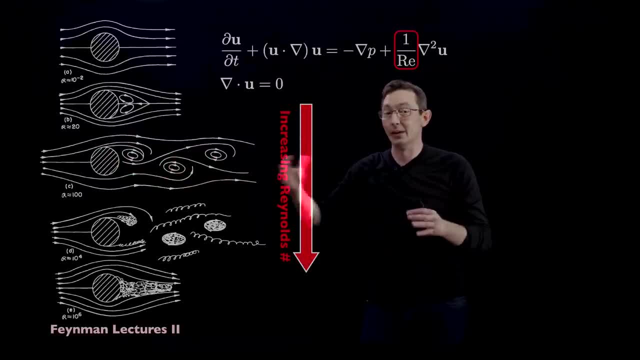 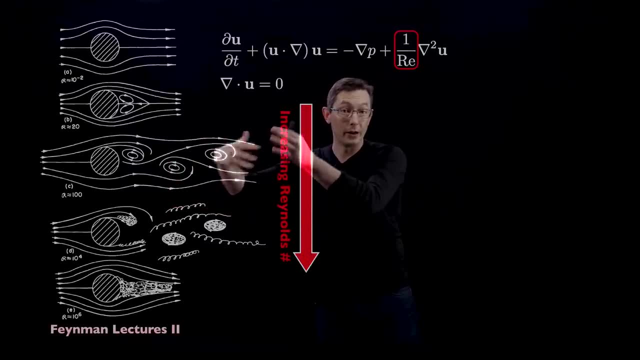 Reynolds, number 100- flow is laminar, So it's not turbulent, it is unsteady, but it's very predictable. So it does the same thing over and, over and over again. It's not kind of statistically unreliable like these turbulent flows in the bottom. 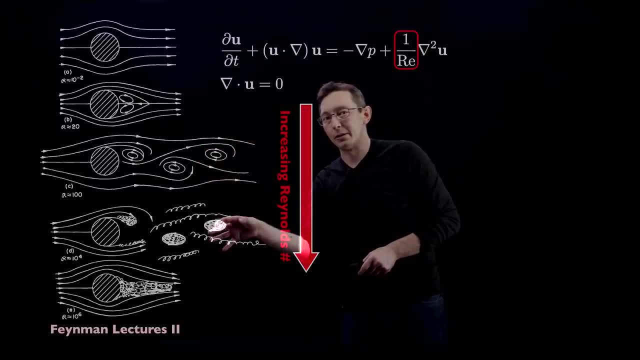 But the middle and the next one are actually very similar. So this is the laminar flow and this is a turbulent flow, but they have a lot of the same patterns and structures, And so what I want to point out is that turbulence is not random. 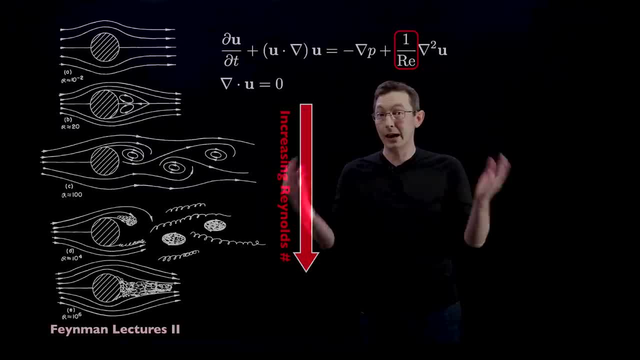 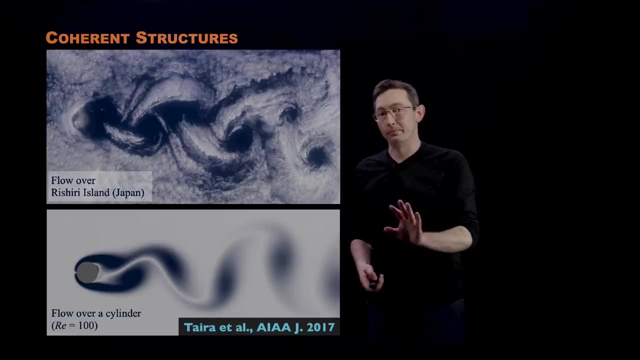 A lot of people think that chaotic systems or turbulent systems are random, And it's true that they have an element of randomness or stochasticity to them, but they are not random, And so, in fact, there are what are known as coherent structures or patterns. 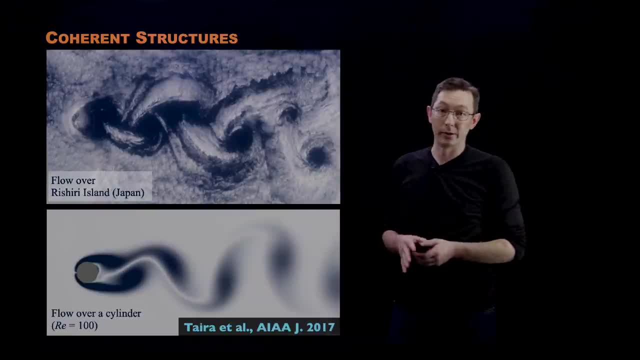 That emerge even in these very, very complex, turbulent flow fields. So this is a picture I pulled from a review paper by Sam Tyra and collaborators in 2017.. I absolutely love this figure. It shows the flow over Rishiri Island in Japan. 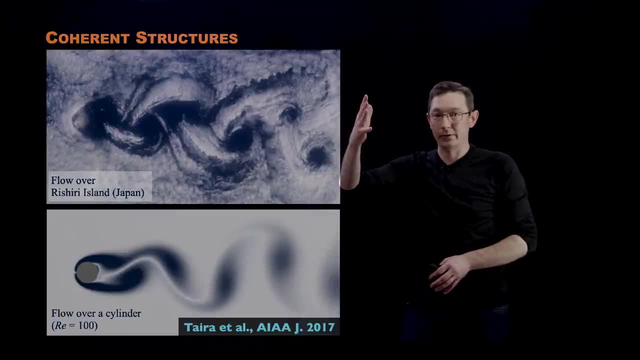 It's literally, you know, the flow over an island. This is an atmospheric flow. And then the very, very simple, laminar, low Reynolds number flow past a cylinder in the bottom. And you can see that, even though the Reynolds number is a very, very simple, laminar flow, 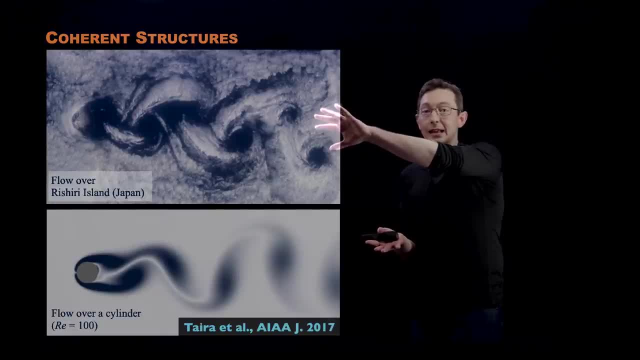 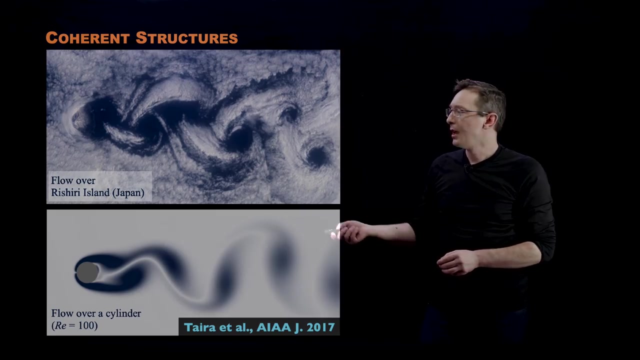 this one's probably in the millions or tens or hundreds of millions, You get the same qualitative patterns emerging in these flows, And so that's really important is trying to understand and characterize those big patterns in turbulent flows. Now I recently saw this video on Twitter and I absolutely love it. 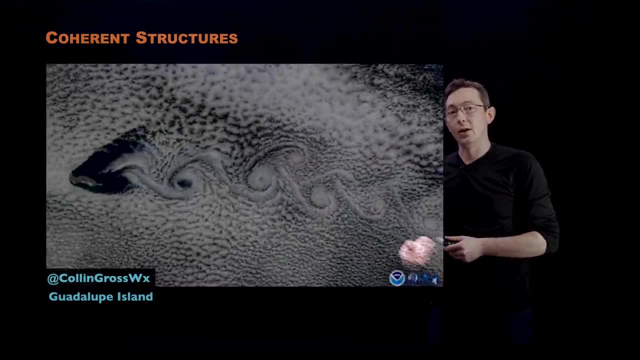 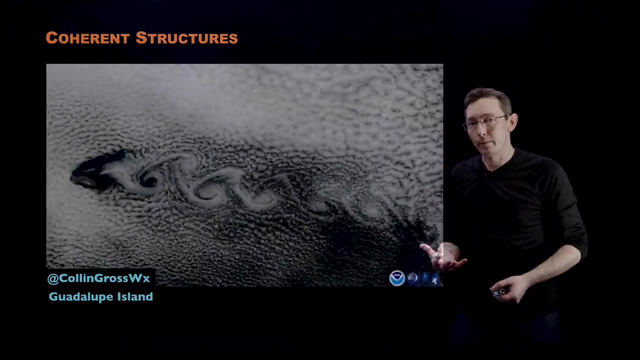 So this is a live video of the atmospheric flow over Guadalupe Island And, again clear as day, You can see the emergence of this Karman vortex street forming in this flow, Even though it's, you know, astronomically high Reynolds number- extreme complexity. 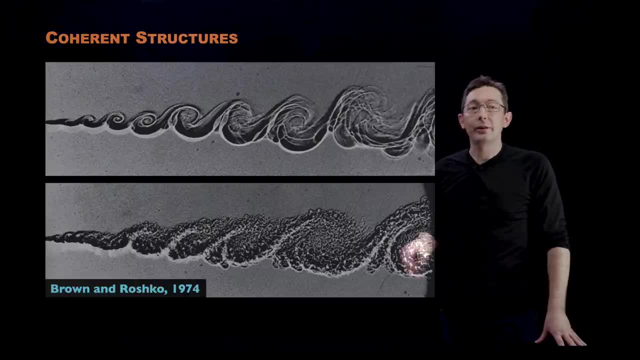 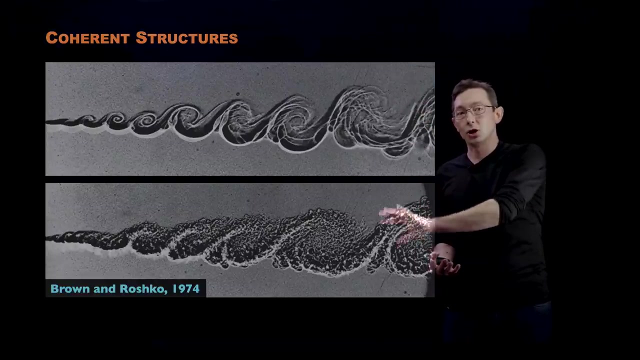 but these patterns, these coherent structures, emerge Now. this was observed early on by Brown and Roschko in 1974 when they were looking at these mixing layers. So these are compressible mixing layers in the laminar low Reynolds number and turbulent high Reynolds number regime. 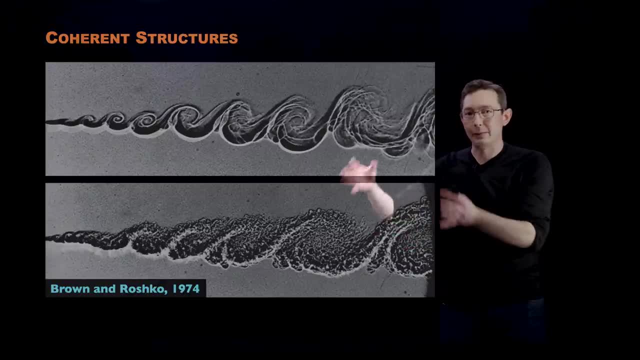 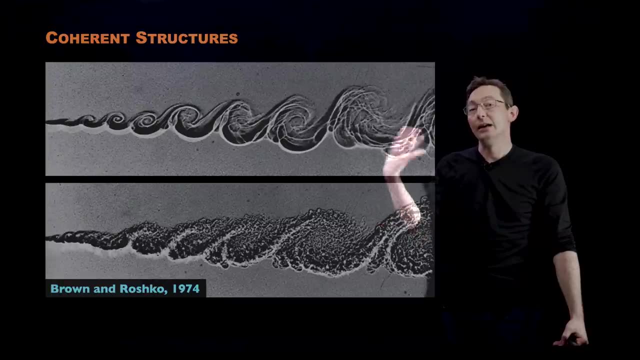 Okay And you can see that. you know, even though the turbulent flow has a lot more complexity and kind of multi-scale behavior, there are a lot of similarities between the laminar and the turbulent case given by these coherent structures. So Brown was actually the other person I learned fluids from at Princeton, Gary Brown. 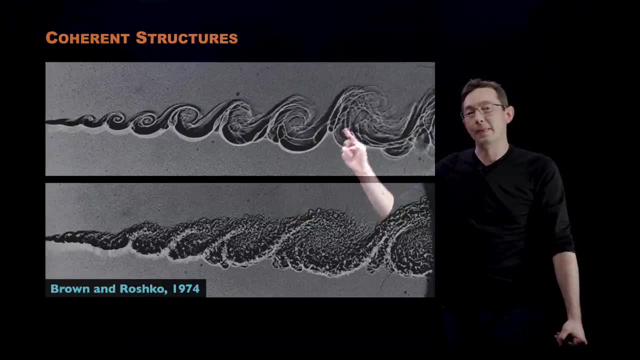 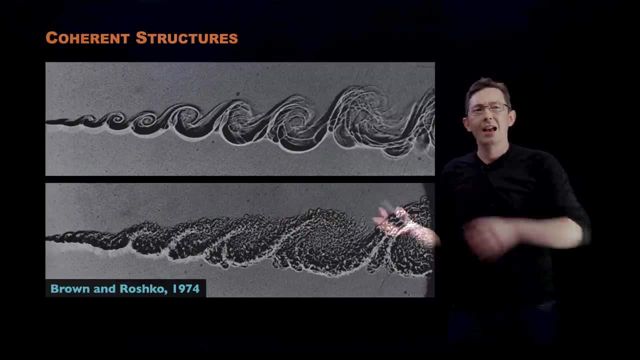 Really fantastic lectures. Roschko- this is not the Roschko of chicken and waffles, although this Roschko also was in LA. I love this picture. This, really this- changed the way that everybody thought about fluids when this picture came. 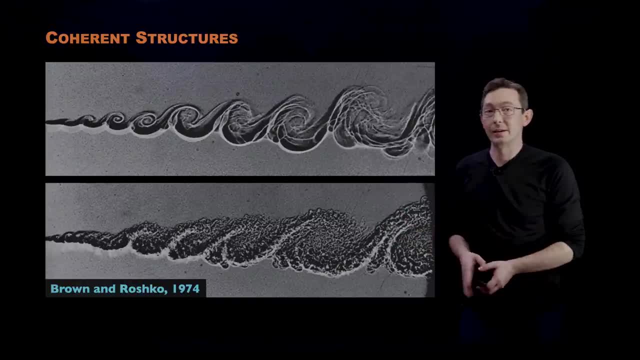 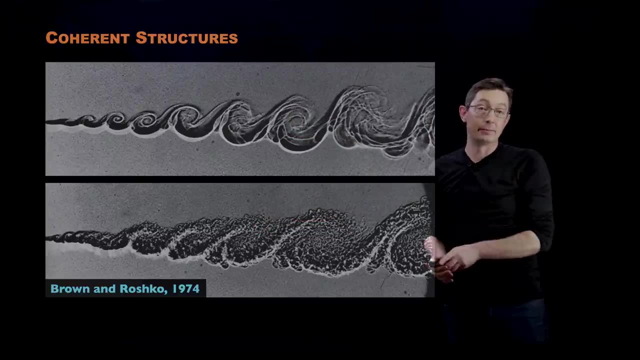 out. It's one of the most famous pictures in all of fluid mechanics because it showed that, even though you have- you know, this incredible complexity, it has a lot of the same patterns of much, much simpler flows, And that really got people thinking about these coherent structures, how to characterize. 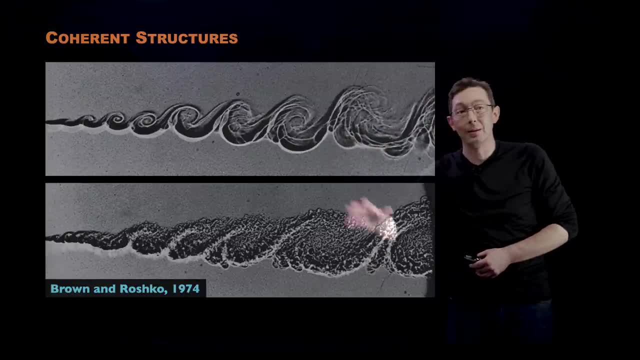 them, how to quantify them, how to model them, And so decades of work, maybe the next, you know, 50 years. up until now, a lot of it's been motivated by kind of this seminal picture. Okay, Thank you. 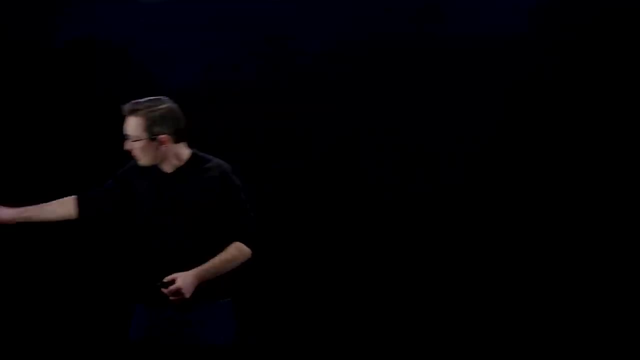 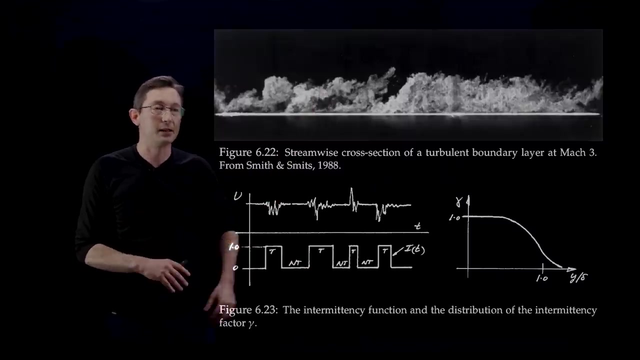 Very cool, Okay, good. So coherent structures exist. We want to model them and characterize them and understand them. Just a couple of other things I want to point out. There's also something called intermittency. I pulled this again directly from Lex Smith's book. 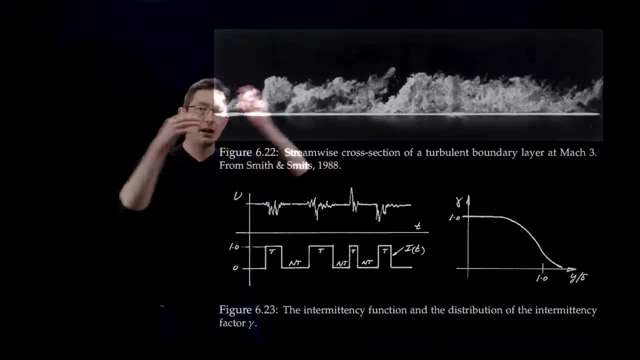 And intermittency. you can kind of picture this if you have clouds that are kind of developing on the planes, as you know, as the ground heats up and the sun is up and you have this wind and this background, It's kind of fun to see how things are going On this boundary layer forming and convecting. 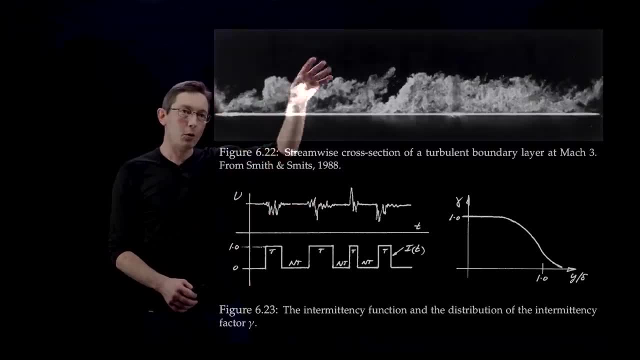 over Earth. some areas of it are going to be more turbulent than others, and some patches you're going to see are actually pretty still. There's going to be patches of still and turbulent and still and turbulent, And so turbulent flows are often what is called intermittent. 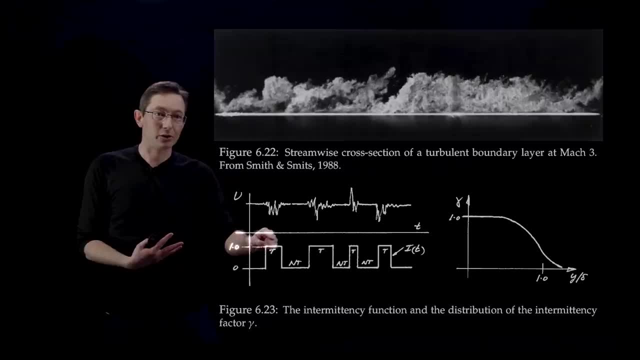 And so you can define this intermittency function which essentially turns on and turns off and turns on and turns off and it tells you when it's turbulent or not turbulent or turbulent or not turbulent. turbulent either in space or in time. that often happens. you can kind of picture if you have a 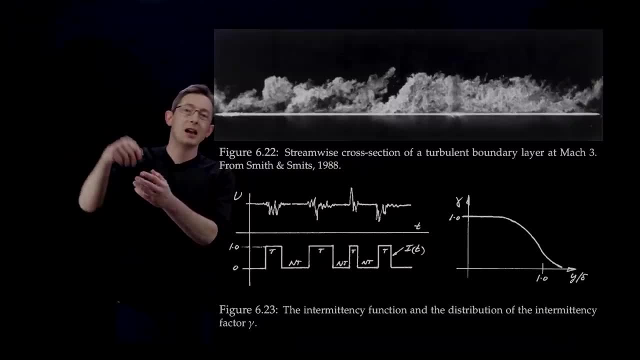 stick of incense or a cigarette and the smoke is rising. you know, sometimes it's going to be pretty laminar, sometimes it's going to be very turbulent. it might actually kind of settle down again and then get more turbulent again, and this kind of intermittency is a hallmark feature. 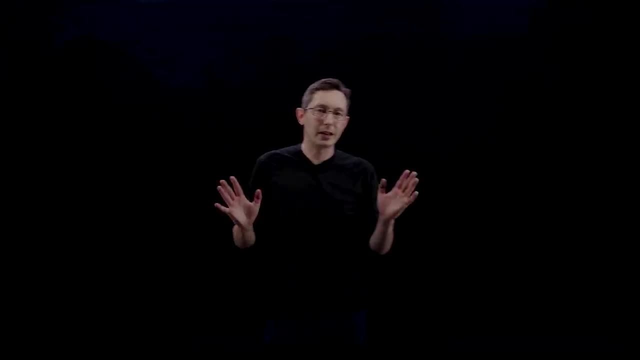 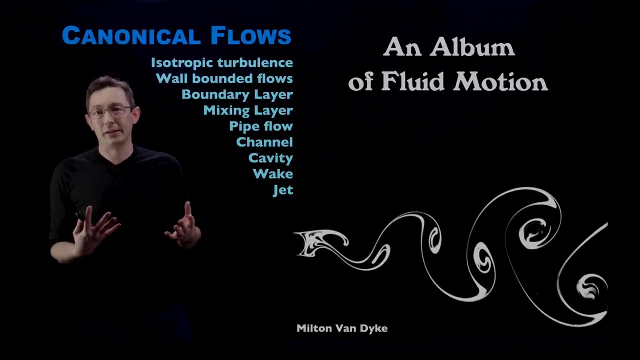 okay. so turbulent flows are everywhere. they're extremely complex, they're very important for us as engineers and scientists, and they have all of these different kind of complexities and features. so how do we get a handle on this complexity? how do we start to model this? now what we have done. 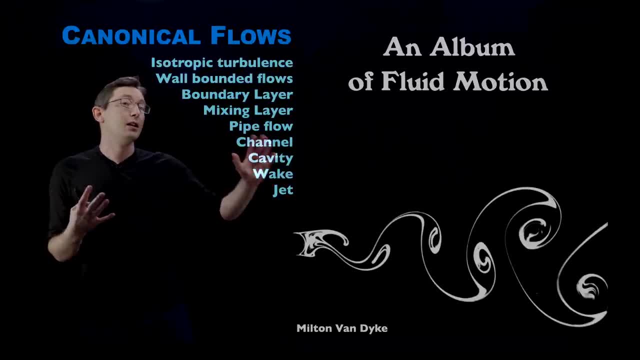 for, you know, the last hundred years since reynolds and probably before, is we've tried to abstract the turbulent fluid dynamics problem into a few canonical flows. simple example flows that isolate the flow of the fluid dynamics. into a few canonical flows. simple example flows that isolate 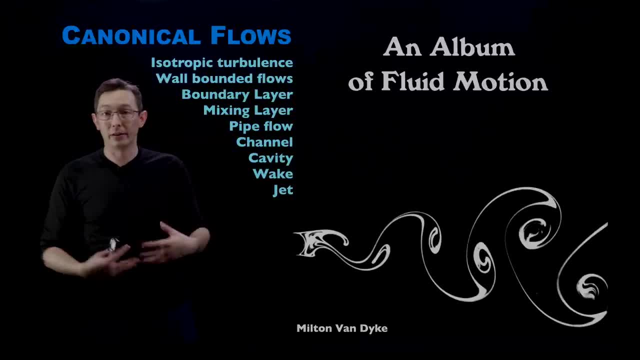 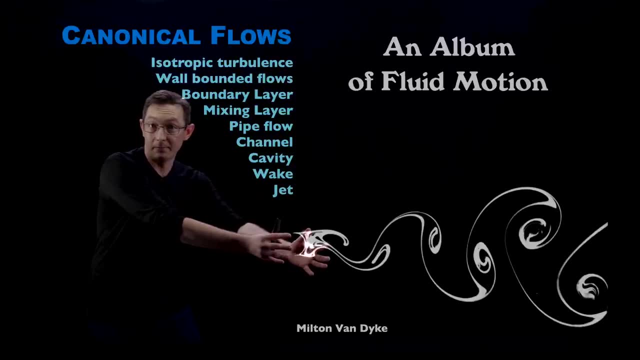 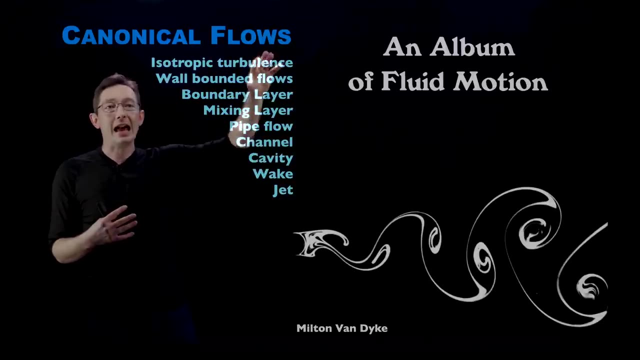 a couple of features. you know one or two features that are that add to the complexity of turbulence, so we can really drill down and start understanding those constituent pieces. now, real engineering flows, like you know, a boeing jet flying through turbulence is going to have a lot of these kind. 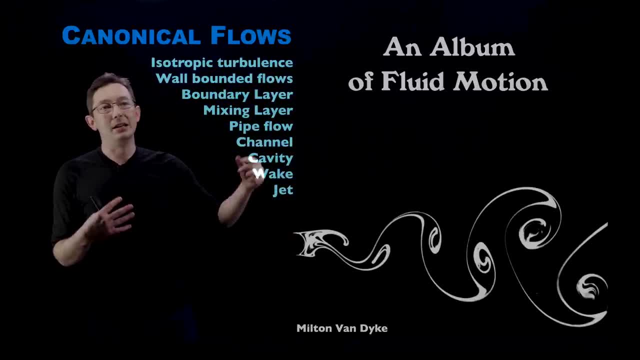 of aspects. you know there's going to be a jet, there's going to be a mixing layer and a boundary layer and isotropic turbulence. there's going to be all of these different pieces working together. but before we tackle those huge problems, we kind of break it down and distill it into. 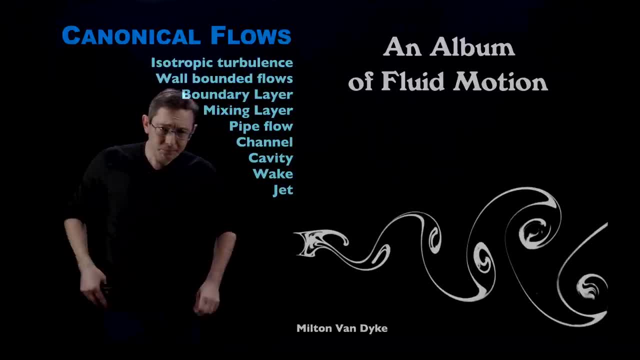 you know isolated kind of idealized problems. there is a gorgeous book by milton van dyke called an album of fluid motion where he walks through you know, beautiful flow visualizations of some of these canonical flows. i think you can find pdfs online. it is really, really cool. 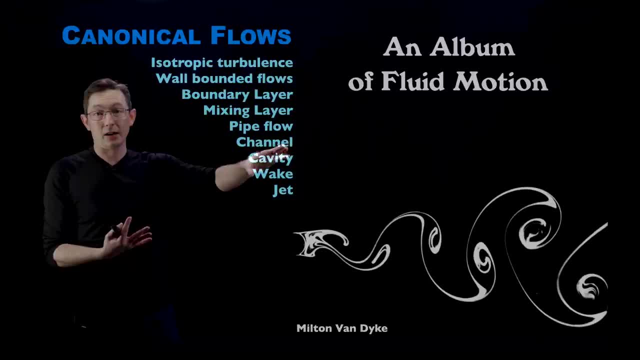 you should check this out. but here is just some of my favorite canonical flows. you know wall bounded flows like the boundary layer, mixing flows. so, um, you know what does the flow behind a wing look like? uh, pipe flows, again pumping, you know, water or oil through pipes, very economically important. 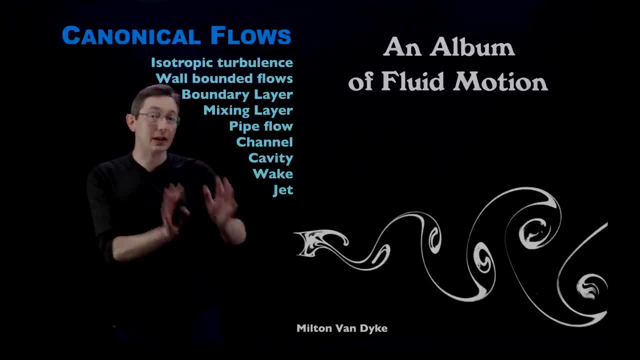 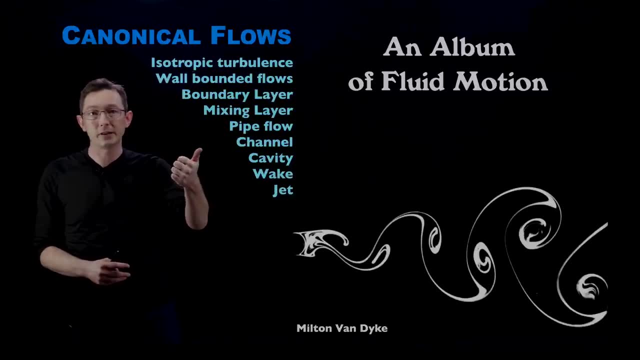 and so on and so forth, and so here i'm just going to go through a couple of these and i'm going to have a whole lecture. the next lecture is going to be all about zooming into these canonical flows, why they're interesting. what are some of the? 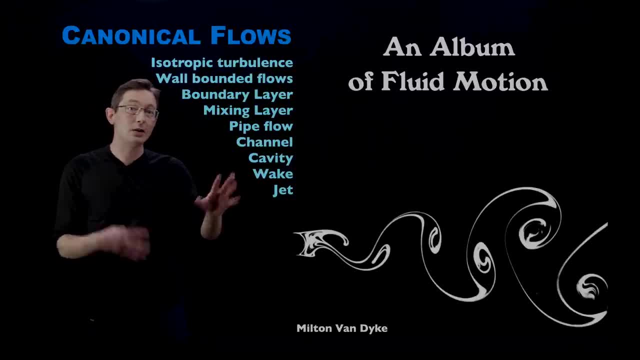 questions we want to ask and answer. okay, but this is how we've approached fluids. uh, you know, essentially for the last century, and this is how we approach most problems in mathematical engineering. where it's too complex is we try to abstract and boil down to the simplest. 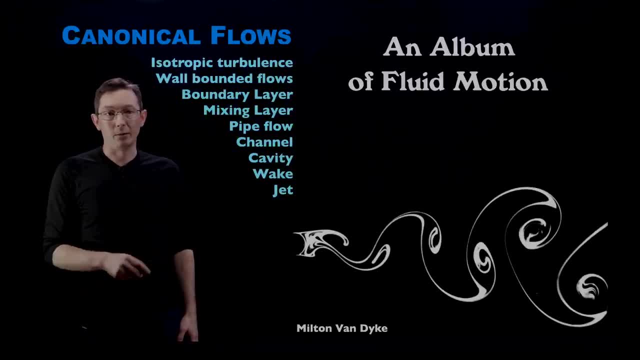 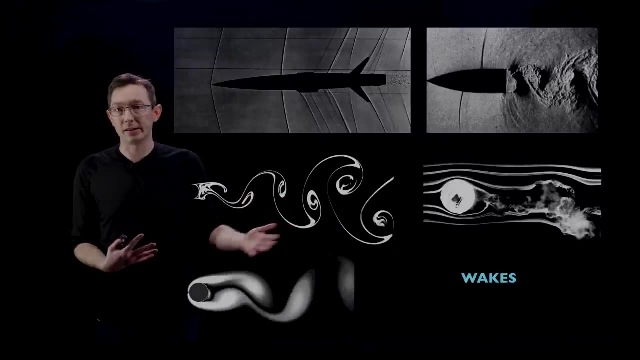 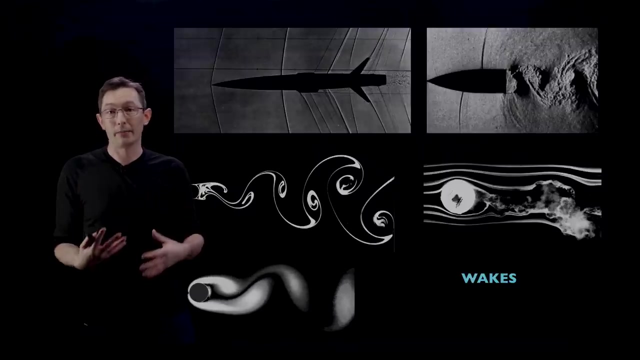 piece that kind of exemplifies our problem. now, calling these toy problems is a little bit, maybe a little too unfair. these are still quite complex and challenging themselves. so just some example: wake flows. tons and tons of effort has gone into studying wake flows. if you want to reduce the drag behind a train or a plane or a truck or a car, you need 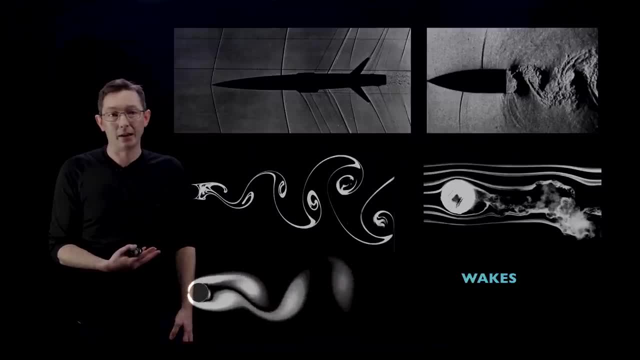 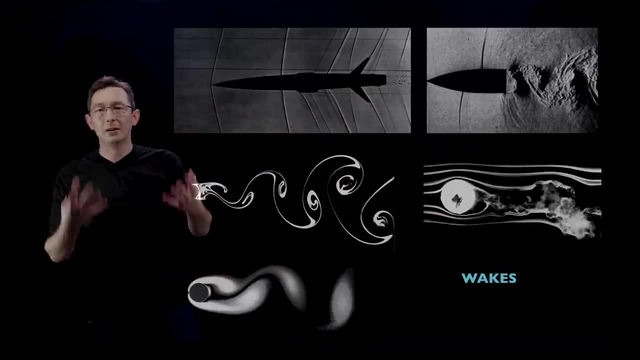 to understand the wake behind behind that body, also hugely important for missile design bullets and ballistics baseballs. you know lots and lots of flows create wakes and those wakes contribute to the drag and unsteady forces on those bodies. another really important example are mixing layers. so again, that broad area is the wave that's going to be the bottom of the wave and we're going to 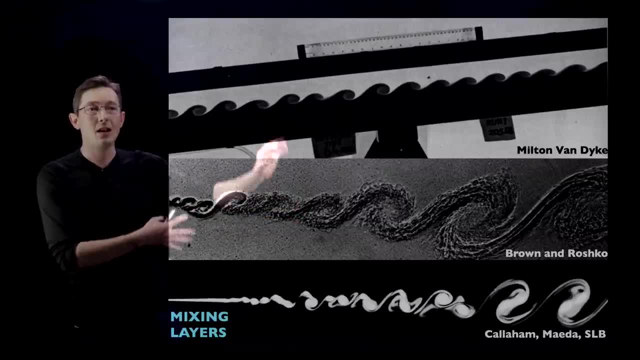 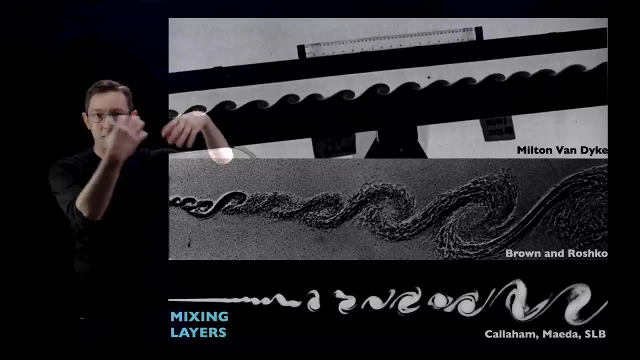 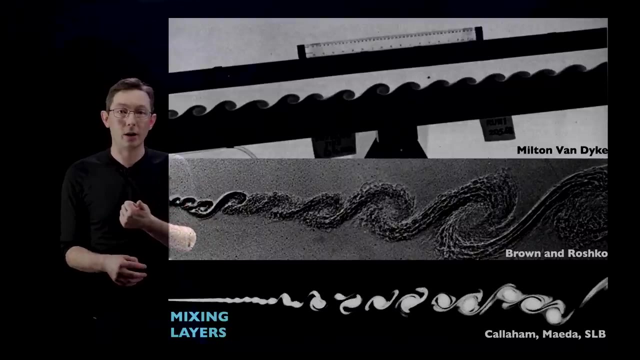 in Roscoe, example I showed, is a mixing layer. many of you have seen these wave makers where you have kind of oil and water in a rectangle rotating and it creates these waves. and these mixing layers are really important canonical flows to understand things like ocean waves, the flow behind a sharp trailing. 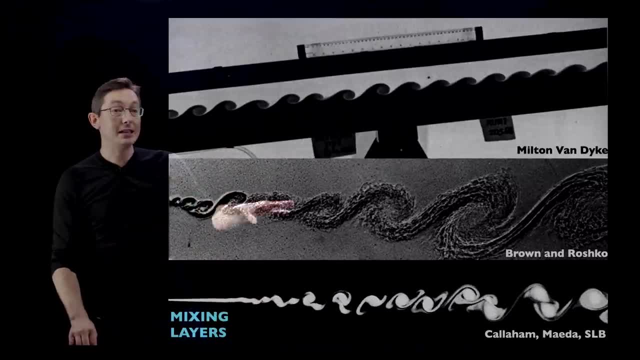 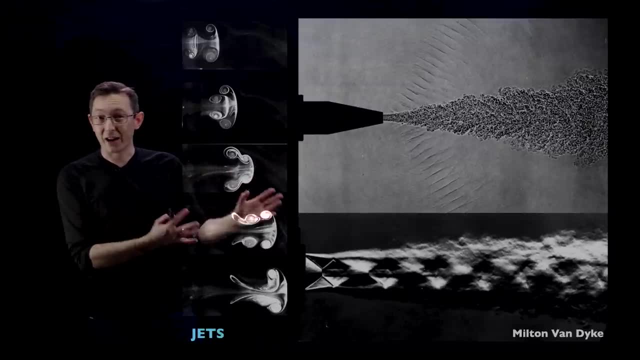 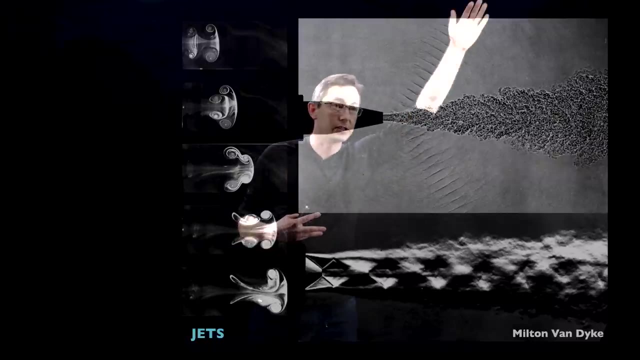 edge on a wing often creates a mixing layer, and these are very, very important. another very important application of fluid dynamics and another canonical flow is a jet, and so there are supersonic jets. you can actually see the acoustic radiation in this turbulent supersonic jets. here you can actually 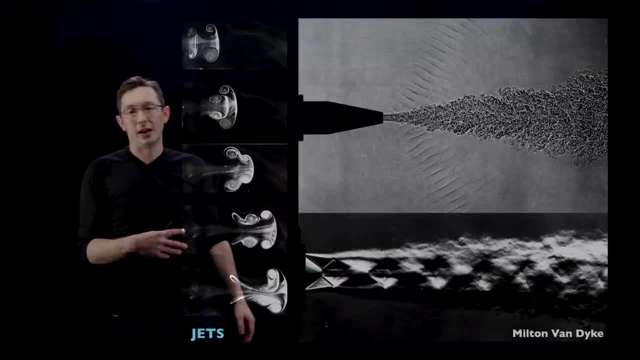 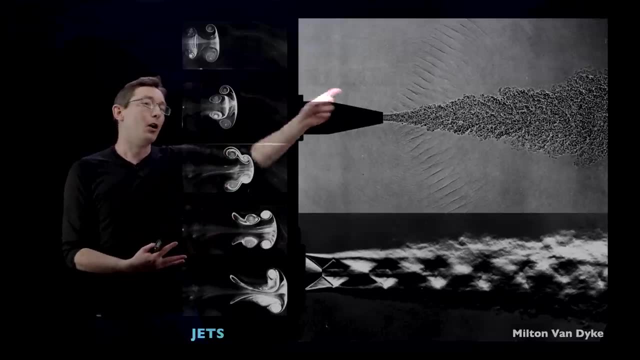 see kind of the mock lines forming in this Jet, and jets are extremely important for you know, producing thrust and power. also we want to minimize the noise, given high thrust, high power. you might have noticed into a譬ight mode of that if you saw the conducive. So you know- any of you who live near LAX or Heathrow know I mean- there's 10 million people in the top two or three airports alone, near the top two or three airports in the world alone that are directly impacted by jet noise. 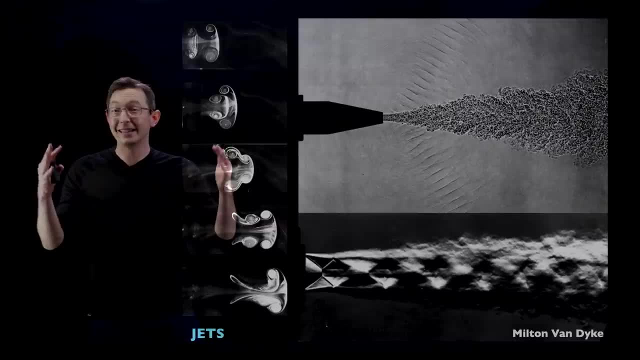 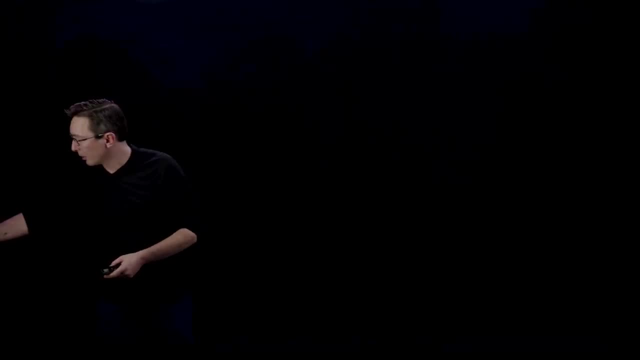 And decreasing that jet noise would improve the quality of life for tens of millions of people directly. Okay so, huge, huge problem here. Okay so, canonical flows are very important. It's one of the ways that we study fluid dynamics. We try to break it down. 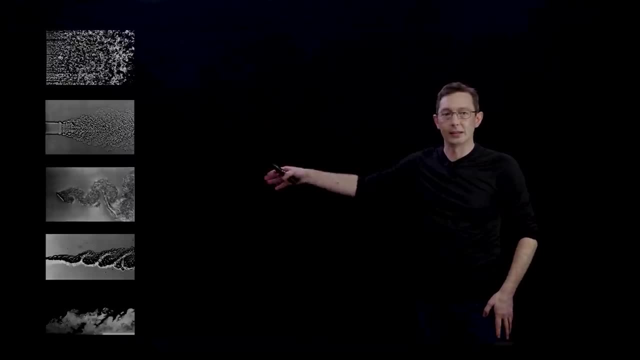 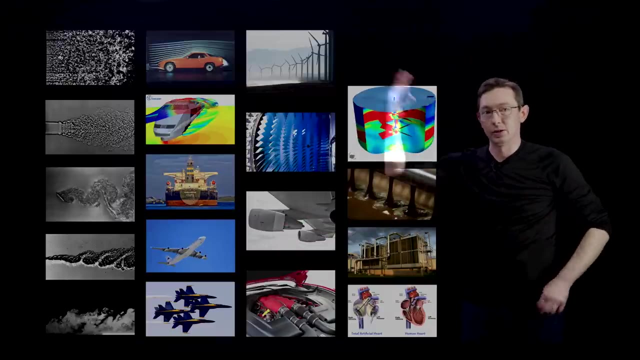 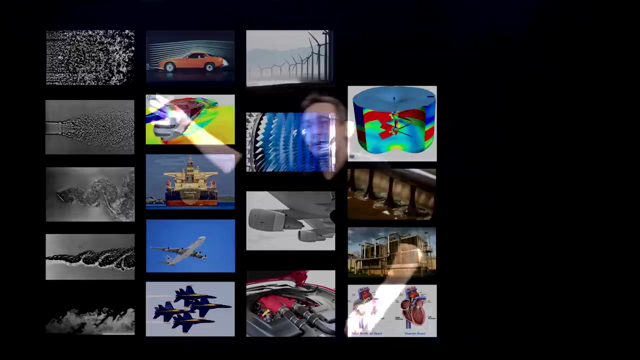 So here again are just some of the canonical flows- wakes and jets and mixing layers- And we use those canonical flows to study much more complex engineering systems like trains and boats and planes and engines and things like that. Okay, so many of these flows are going to have lots of elements of these canonical flows. 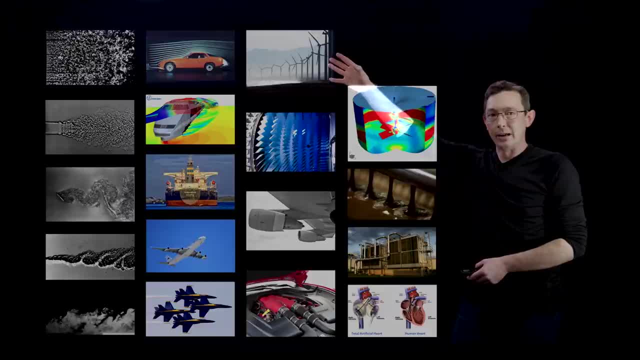 And I'll talk about that later. So, for example, you know, a wind turbine, There's going to be boundary layers and mixing layers and wake flows, all of those interacting in a pretty complex system And, at the end of the day, we want to understand these systems. 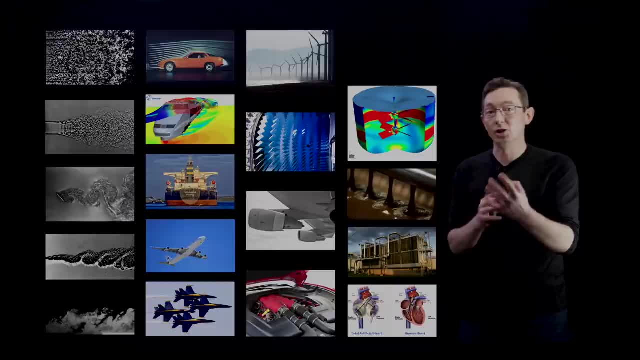 We want to be able to model them and understand what they will do when we change different things about our engineering designs. That gives us the ability to optimize, for example, design better blades for turbines, but also to control the system, to actively manipulate the behavior of the fluid. 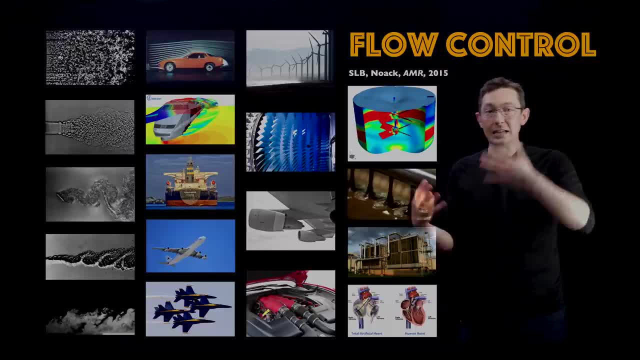 For better engineering outcomes: to increase, lift, decrease drag, enhance mixing, things like that. Okay, and this is something I'm very passionate about And one of the reasons I love turbulence, as you know, an important field of fluid mechanics. 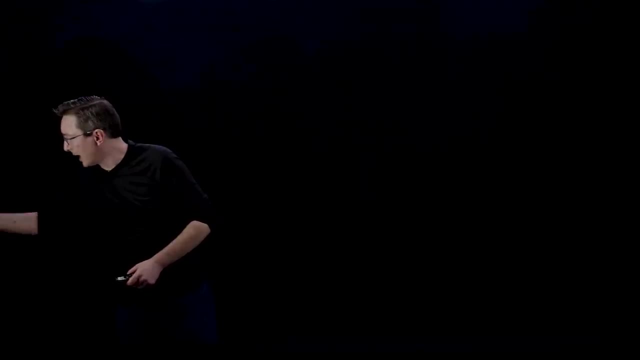 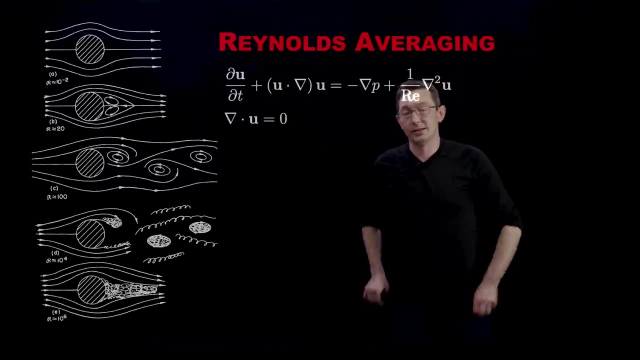 Okay, good. So I think one of the last things I want to point out here is, again, we go back to this. We're always going to go back to the Navier-Stokes equations. That's kind of our entry point as mathematical engineers. 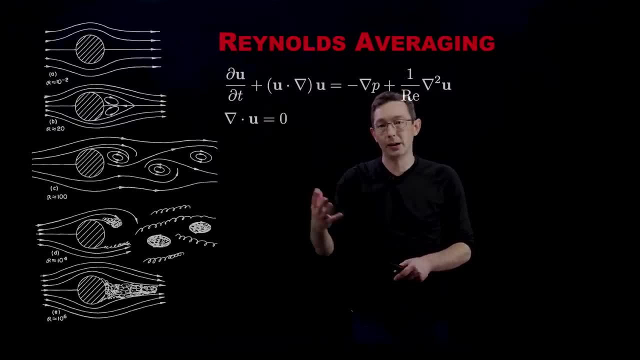 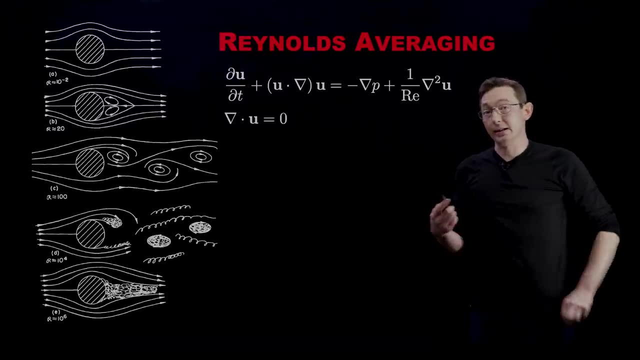 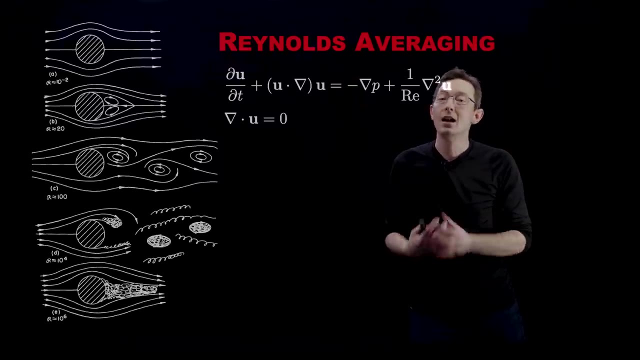 And we know that we have this kind of increase in complexity with the Reynolds number. So one of the kind of important things that you can do to study these flows- and I'm going to have a whole series of lectures on this- This is going to be the basis of what's known as turbulence closure modeling, which is one of our approaches for modeling these systems more efficiently on computers. 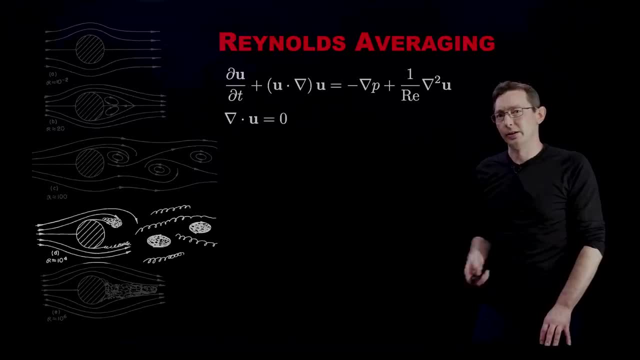 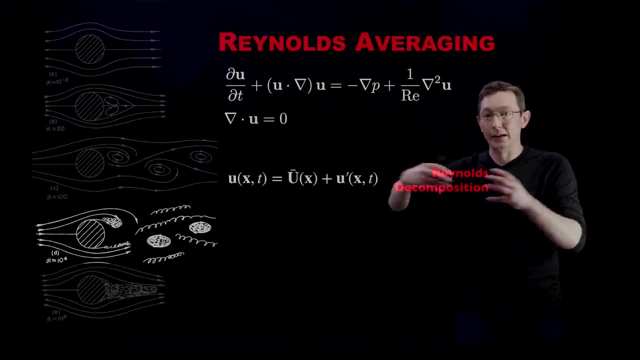 One of the things you do if we zoom into a turbulent case is something called the Reynolds decomposition. So we're going to take this flow field U, which is, you know, a very complicated function of space and time, and what we're going to do is we're going to break it apart into an average field, U-bar, and all of the fluctuating components, U-prime. 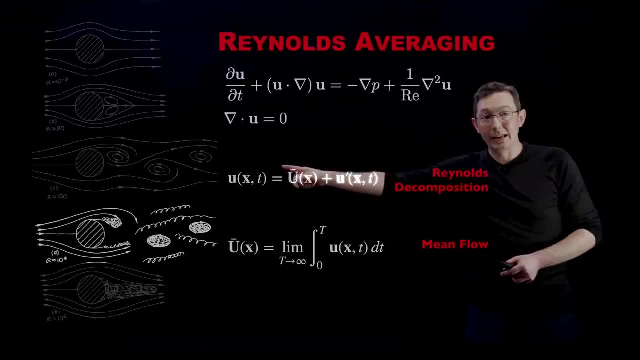 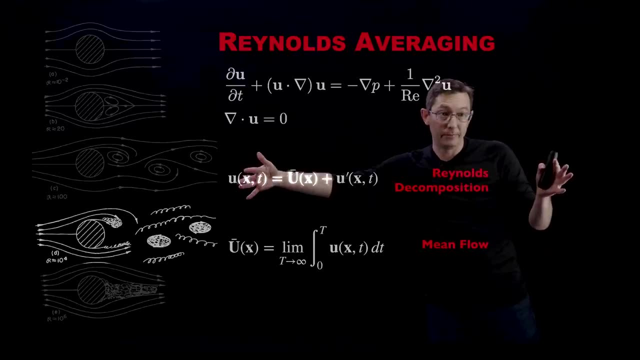 And so, U-bar, we get by literally taking this flow U and just averaging in time. we just take flow snapshot. think of a movie, of this flow evolving. I'm just going to average all of those frames of the movie in time and get the average frame. that's the mean flow. 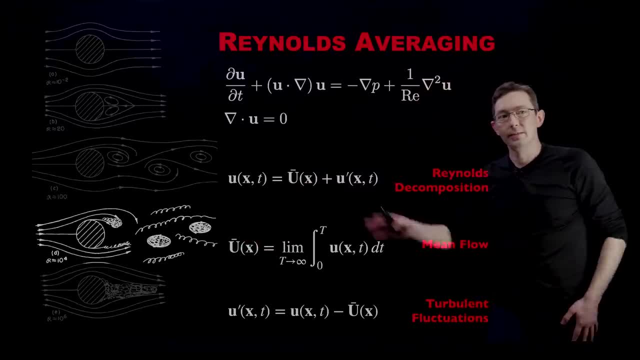 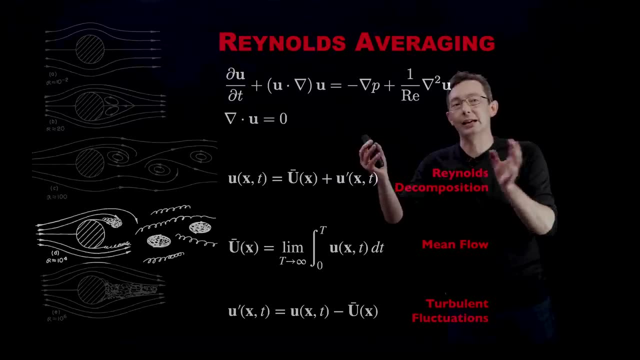 Okay, And then the turbulent fluctuations are just my original flow minus the mean flow. Okay, And so what we're doing is we're taking our flow and we're decomposing it into a function that is the average flow, which is no longer a function of time, it's just a function of space. 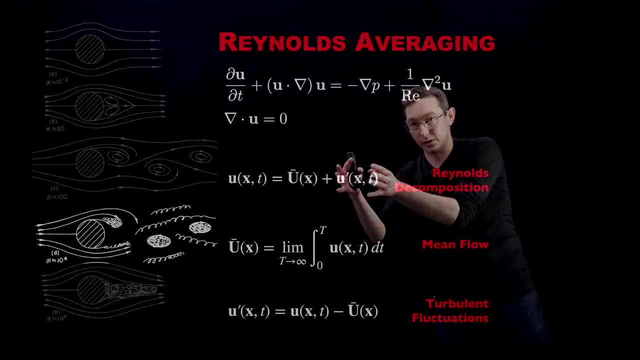 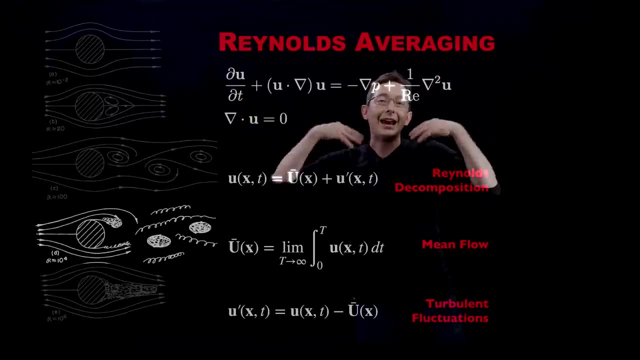 And then all of these little fluctuations, all of the turbulent fluctuations, And when I take this decomposition and plug it into the Navier-Stokes equations, I get lots of interesting things happening. I get an equation, A Navier-Stokes equation for the mean flow and for the fluctuating components, and I can model things more efficiently this way. 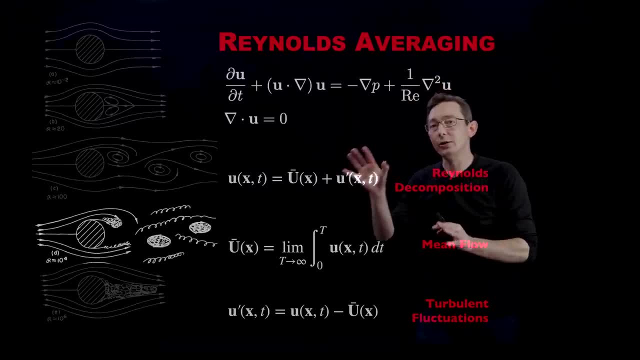 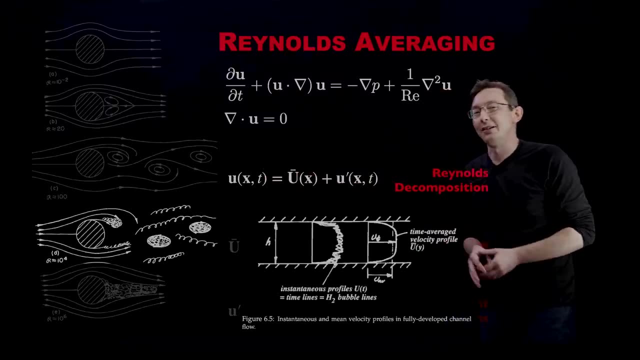 Okay, So huge field of Reynolds averaging. but this is a very useful perspective where we decompose our flow into the average flow and the fluctuations. And I'll point out this is largely historical. why we do this- and it's kind of fortuitous- is that historically we didn't have computers to measure these flow fields accurately. in this, 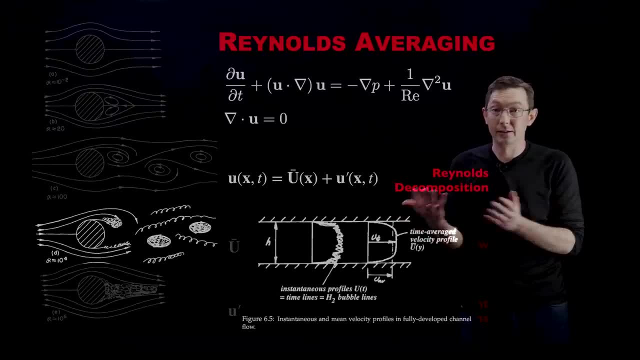 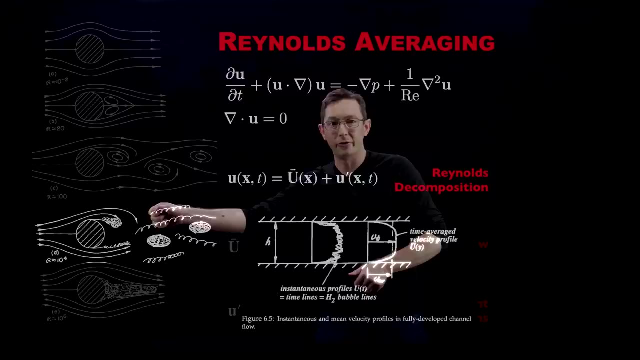 space and time. we didn't have laser technology until the 60s, 50s and 60s so that we could build laser sheets to image the full flow field and experiments. and so back in the olden days you were stuck with single point measurements, hot wires, where you would put a hot wire in the flow. 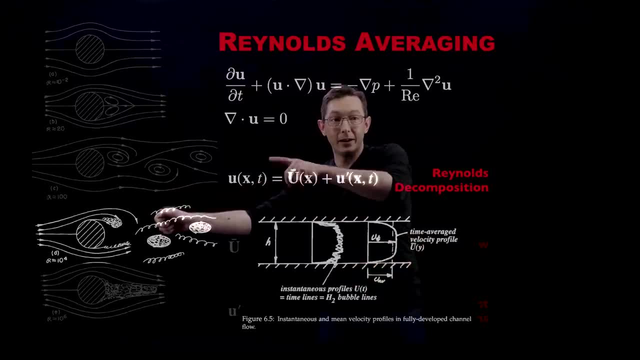 and i could maybe measure that for a long time and figure out what its statistics were and average and build the fluctuations and then i could move it one delta x or delta y down and then i could move it again and move it again and in the course of a day or a few days i might be able to measure. 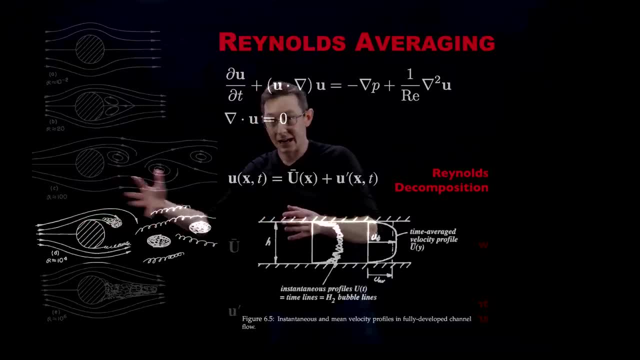 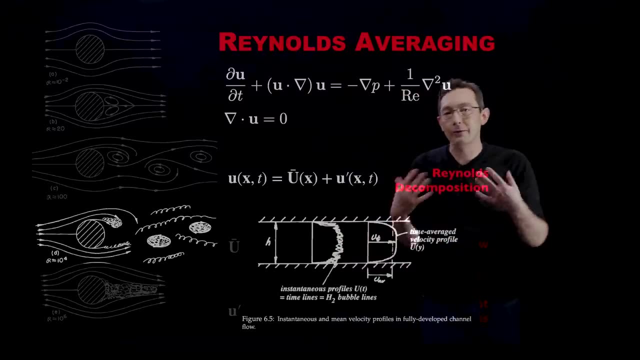 the entire wake, point by point, in a time series fashion, but i can't tell what every point is doing at the same time, and so this idea of averaging your flow is actually, you know, goes back to the days when we didn't have enhanced measurement techniques and computers, but it 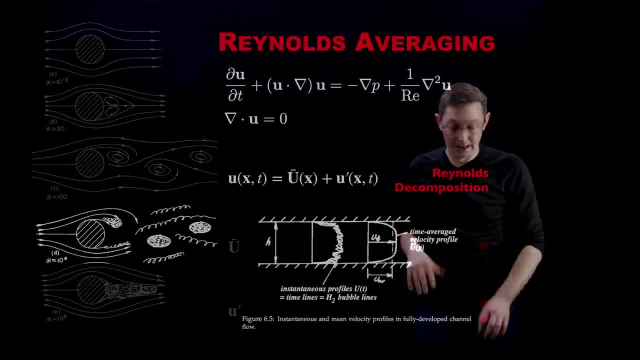 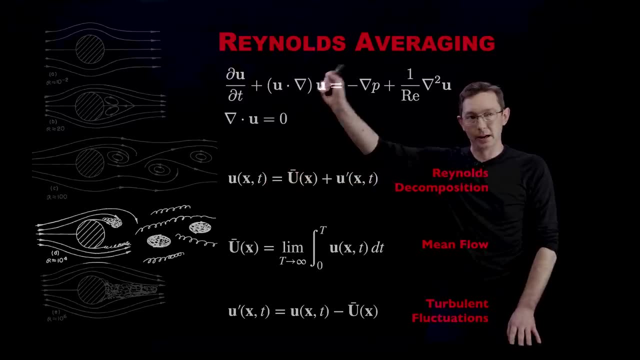 turns out that it's a very, very useful perspective for modeling today, so that's pretty cool. okay, good, so i'm going to have a whole lecture on reynolds averaging soon. this is going to be kind of a pen and paper or like light board video lecture, and i hope that i have convinced you in.